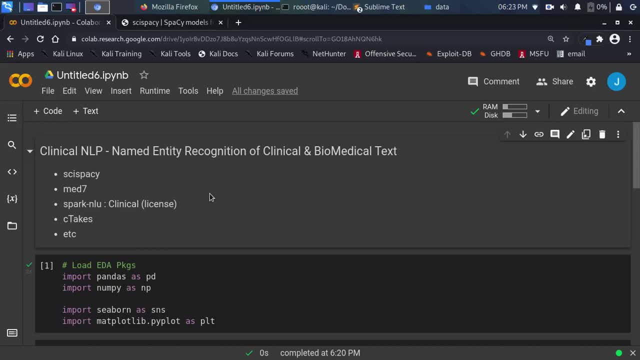 Alright, so welcome back again. my name is Jesse and in this wonderful and exciting tutorial we're trying to see how to do named entity recognition of clinical and biomedical tests. so this is a format of clinical nlp. so in this tutorial we're trying to see and explore some. 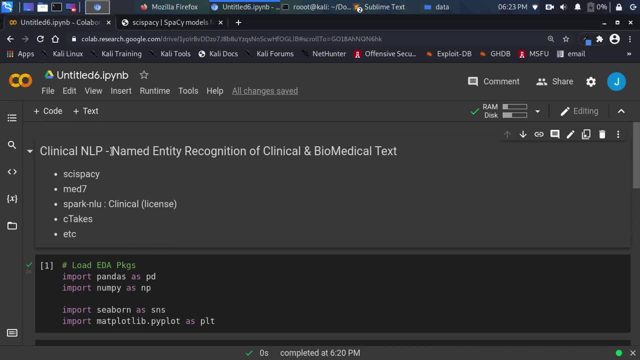 libraries that we can use to do clinical nlp right, especially specifically named entry recognition. so one of them is cyspacey right, which is very powerful for doing clinical nlp as well as biomedical nlp. we also have med7, so med7 and cyspacey all are libraries that depends upon. 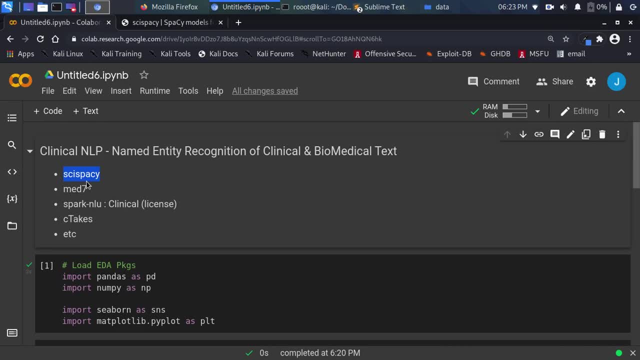 spacey right. so the pre-trained model that you can use together with spacey spark nlu is built on top of spark, which is very, very powerful by just no labs, and it's having a clinical version which you require a license or an activation key to work with because it's a software you must buy right. 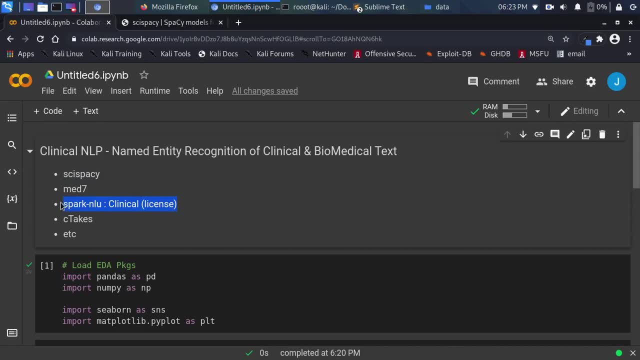 it's very, very powerful. it has some very cool features and understand the reason why they need to. you need to buy for the because it's very useful, very powerful. and there's also ctex and nrs. so let's see how to use cyspacey mh7. then another tutorial: we'll see how to use spark nlu, the clinical version. so i'm going. 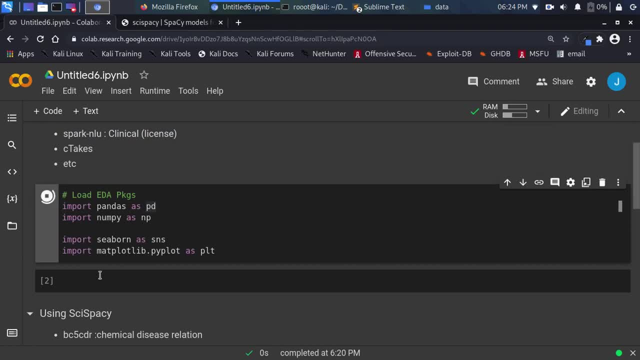 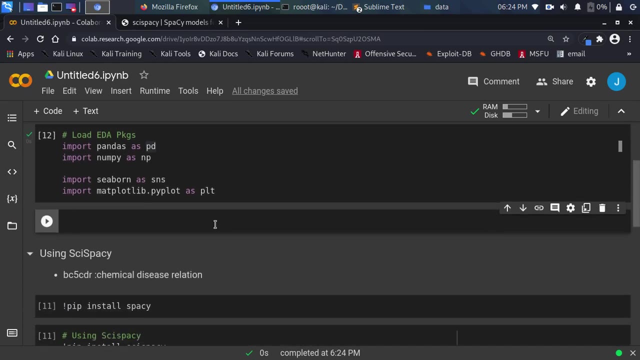 to load my eda packages and then my plotting library. then you'll be loading our data set. so the data set you're using is a medical data set from here which consists of several medical history, together with the disease and a description. so i'm going to load that data set. so let's load the data. 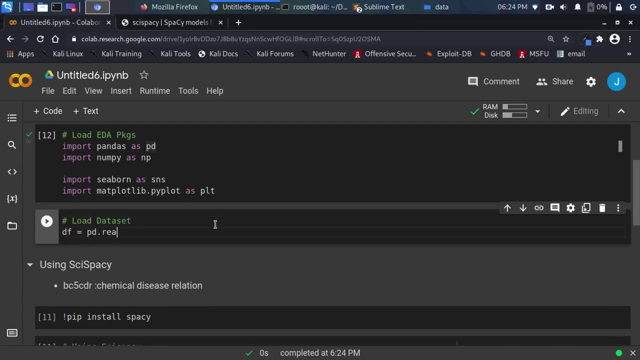 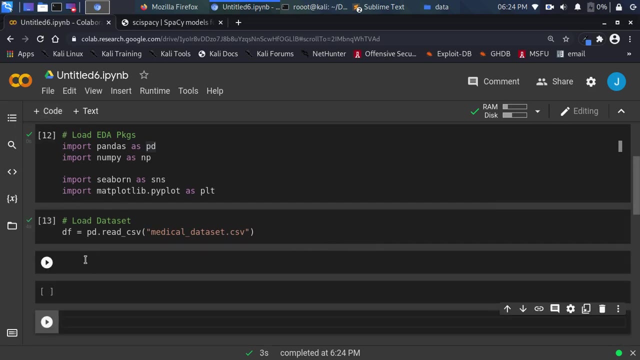 set. so let's go to the dfpd, read underscore csv- my medical data set, dot csv. so let's open this and then let's explore this particular dataset. so we're going to load the dataset and now we can explore it. so let's check it out. so if i go to dfhead, we can see that this data set has several 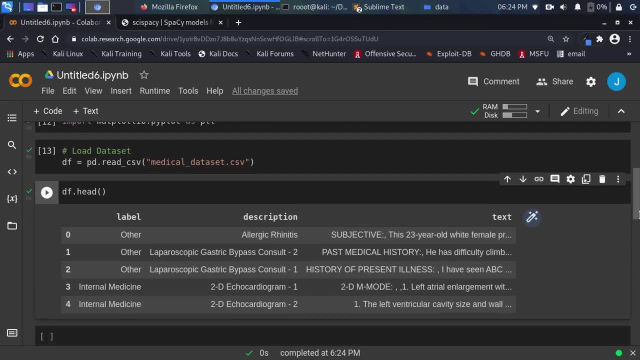 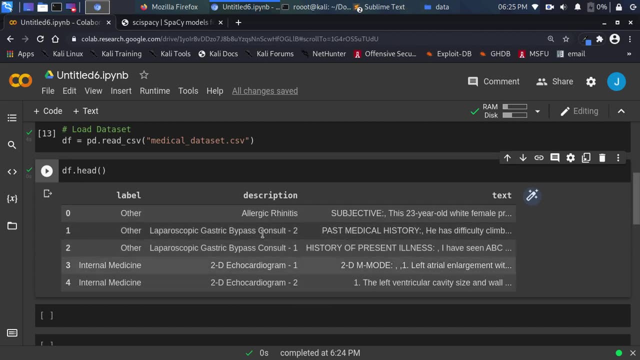 tools, several features. so we have the label right, which have several maybe in the future to do some test classification. we also have the description of the particular diagnosis and we have the test which is the medical history. so we'll be picking this particular one to extract clinical named entities from it. okay, so let's see a simple example. so i'm just 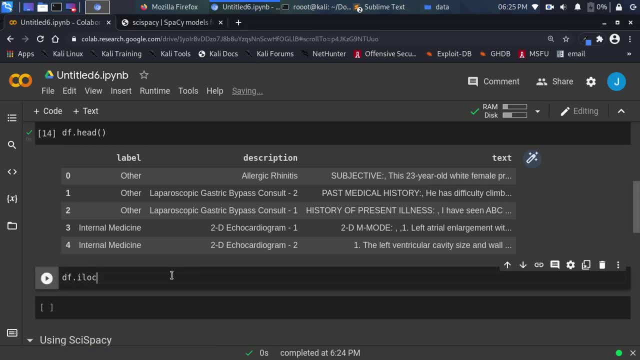 going to pick one. so df dot, i look and now let's say let's pick um two. right, then if i pick the test column, you can see what we have. so, based on this simple data that we have, we have several things there. right, you have the history of presenting on us and i'm doing this, right. 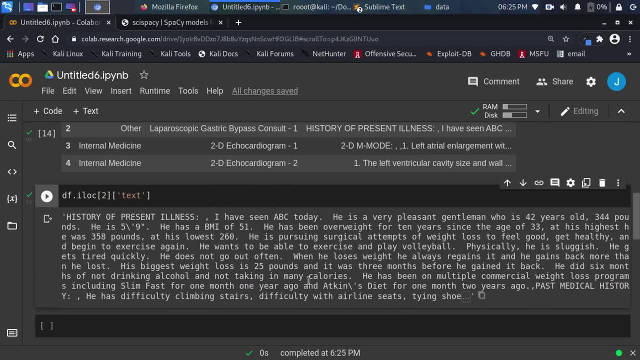 and then we have the bmi. we have some, some information there, so we want to be able to extract if they are medical or they are biomedical named entities within them, right? so that is one of this. if i go back and i pick one like this, you can also see a different one, right, with different. 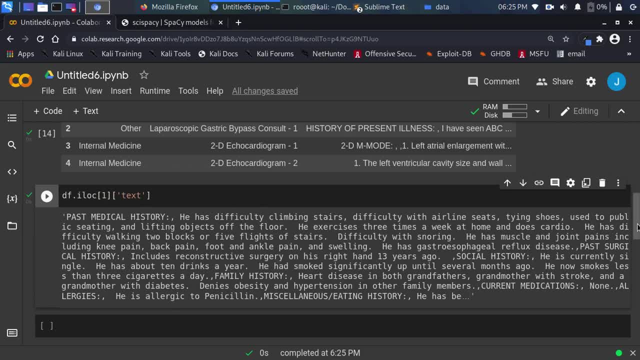 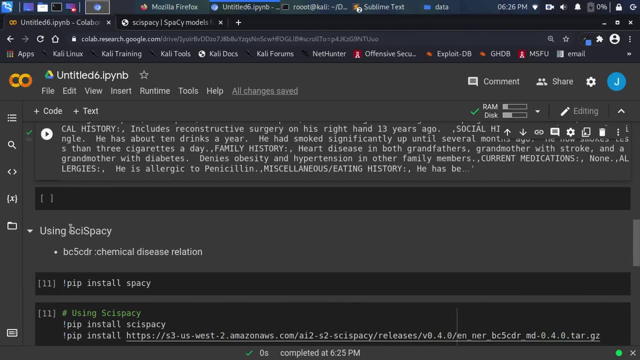 things that we can pick from. okay, so let's see how to work with this so busy inside spacey, then later i'll use match 7.. so first of all, in case you don't have the information that you want to use size spacey, you will have to install it and then size size spacey depends on space you have to. 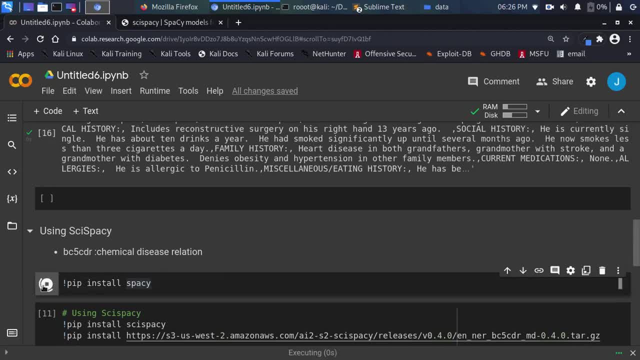 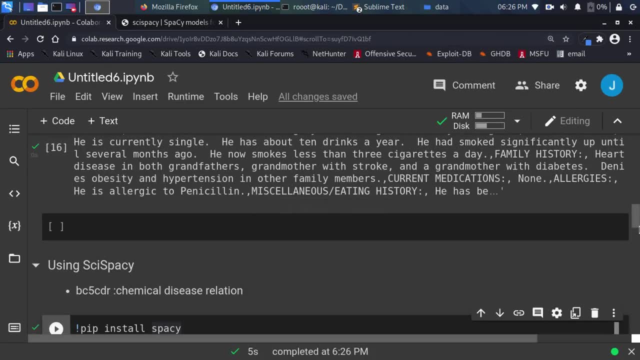 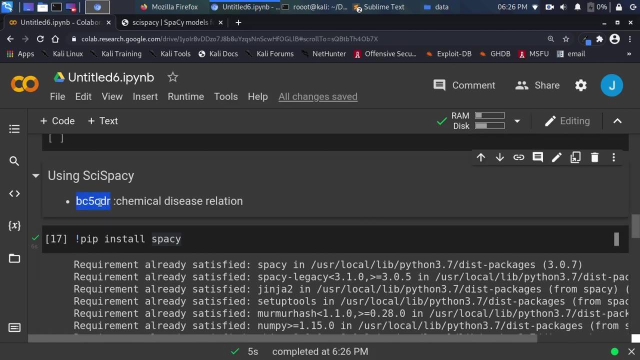 first of all, install specie, so pip, install specie to install size specie, as the first thing you need specie, and then so that we also need to be installing size spacey, right. so we size spacey gives you several pre-trained models that you'll be using. so we're using the cdr, which is a chemical. 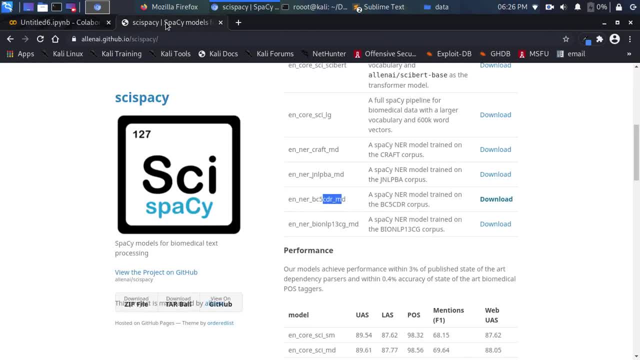 disease relation model. so i get all the various models from here to size allen, size spacey, right, allen aigithubio, size spacey, and you have several pre-trained models there, right? so different models there. so you need to install it- this how to install it- and then you pick the. 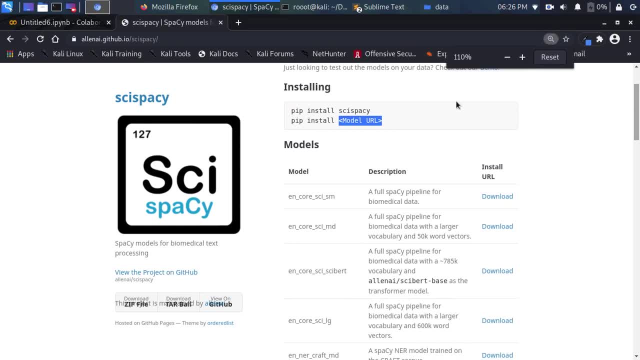 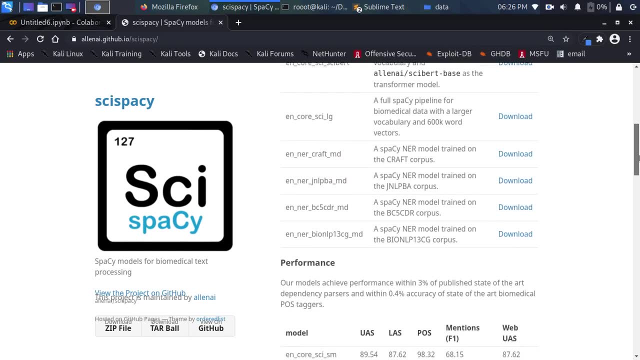 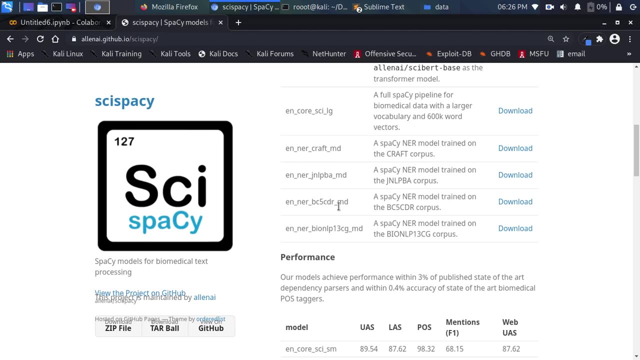 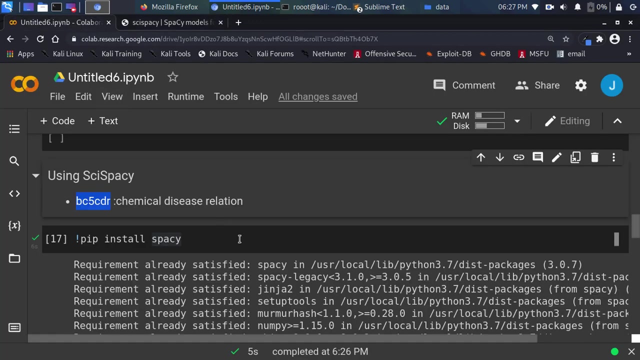 model. then you install it. so i just come back. sorry for it being small, perfect out. so these are the different models trained on different data. so i'll be picking the bc5, bio creative, cdr, chemical disease relation medium database. so i just click on this and copy link address: right, i go back again, then let's install it. so to install it. 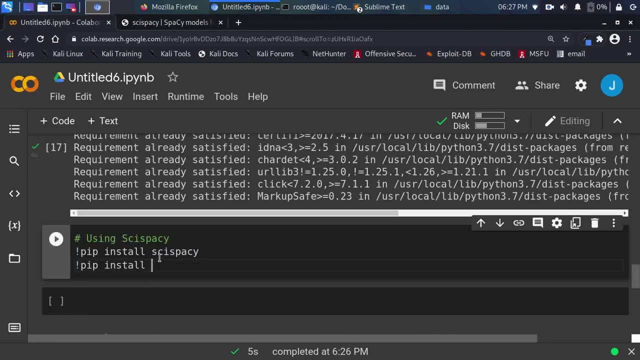 it's just very simple. so just go with: pip. install size specie, right, then pip. install a paste in the url i copied, right? if i paste in the url, you can see that the same url that we have right and this is the particular model we'll be using. this is the name. 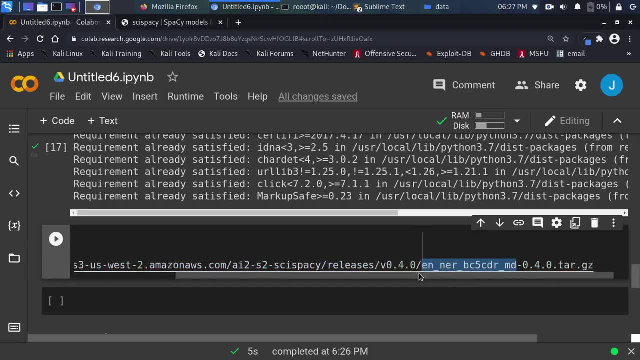 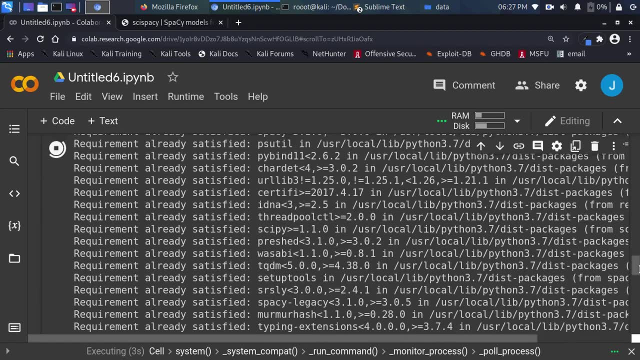 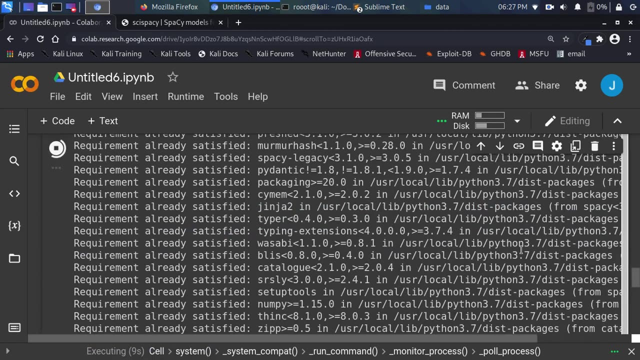 of the model, right? so this is what you use. so let's install this on our system. so i click on it to install it. so requirement already satisfied, because i've already installed it before. it's collecting it from here. so this is going to be the pre-trained model, right? so there are. 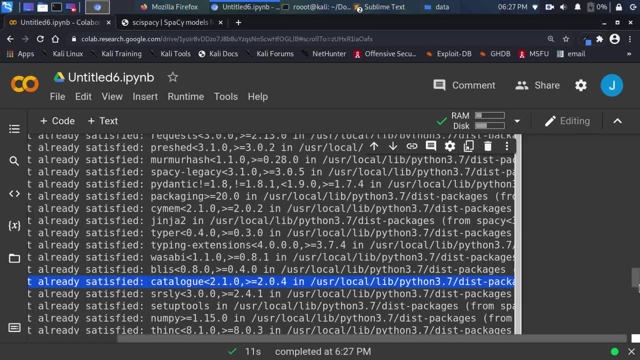 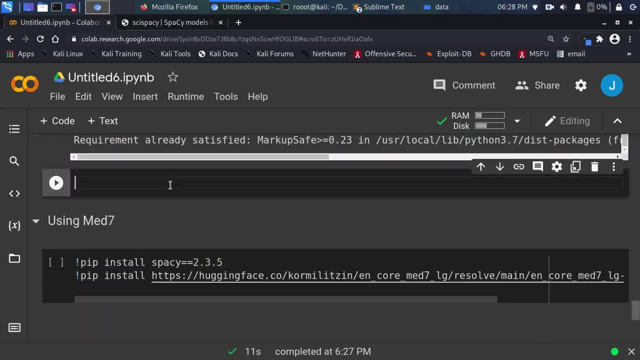 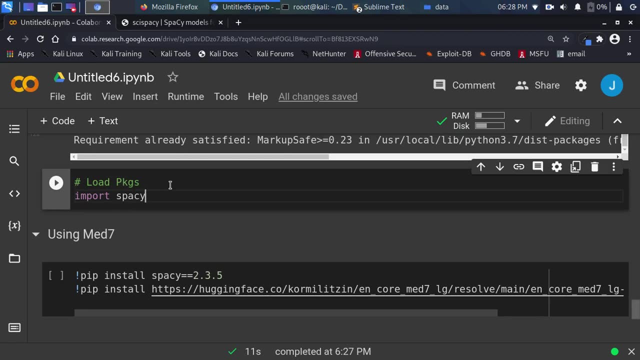 several models you can use to do your work. right, we still need a test. okay, perfect. now let's go back and let's see some things you can do. so, first of all, let's import the packages. so we'll be loading the packages, so we're importing spacey, and then you also import. 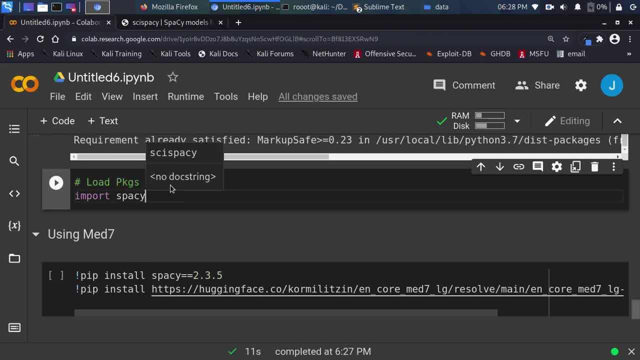 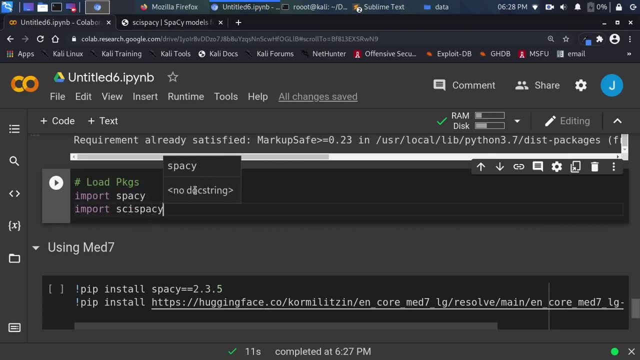 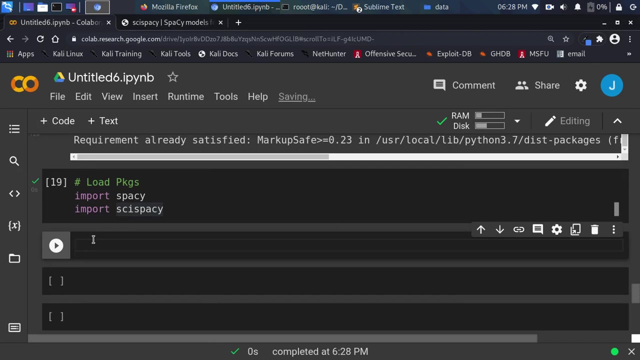 import spacey and then also import size spaces. so import size spacing, right. these are the twitter stuff you may spotted, so let me put these two perfect. and now let's create our nlp object and then see how to do clinical nlp, or clinical named entity recognition, on our data set. so to work with it, just go with, let's create our nlp object. so 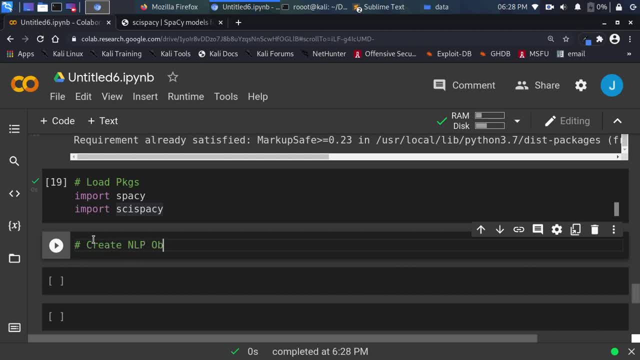 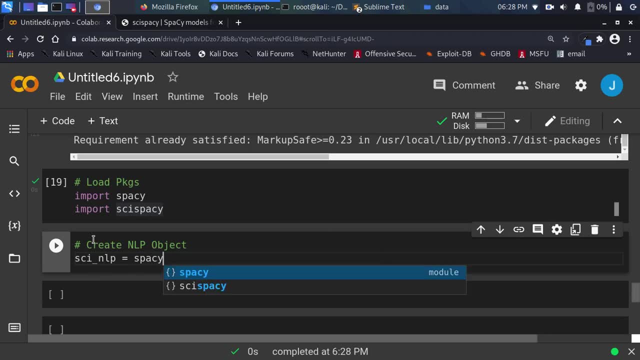 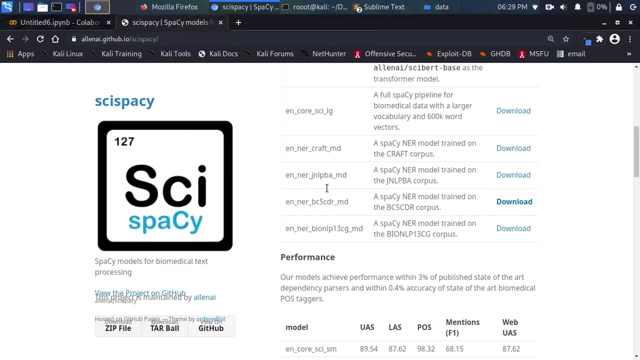 this is going to be my size nlp, which is going to be my specie dot load, and i'll pass in the name of the model, right? so this is the name of the model, which is the same name we had here, right? this name, that's what i'm picking, so this particular name is what you are picking as this, right the same. 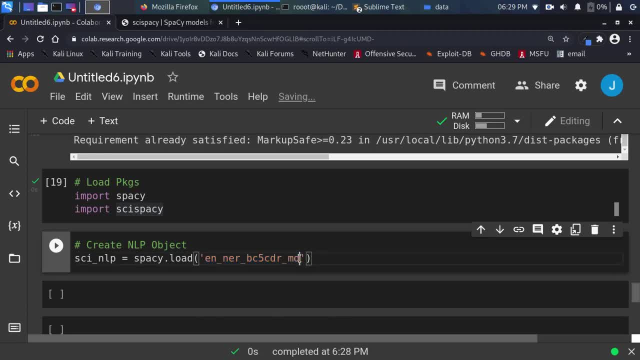 thing we have here, making sure that the same perfect. now this is going to create an nlp of a object with the pre-trained model- not the normal default english that we use, but with this particular pre-trained model. then let's explore the various component of this model. so this is: 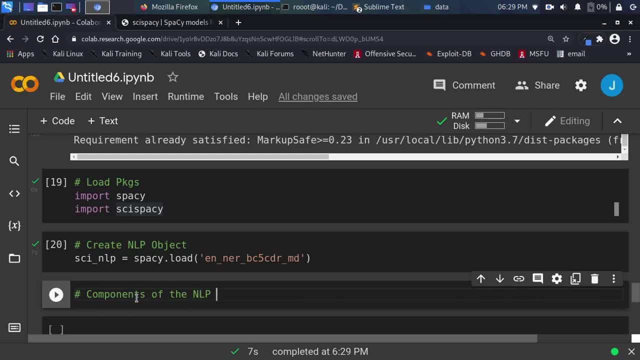 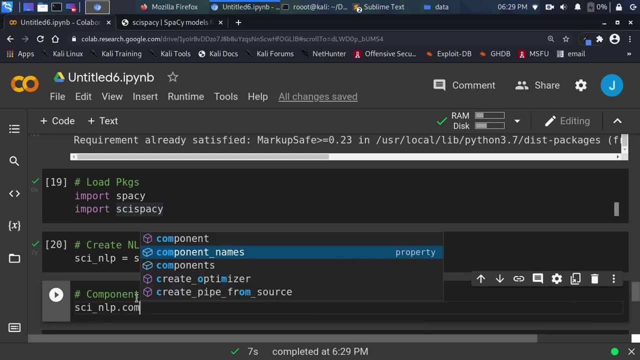 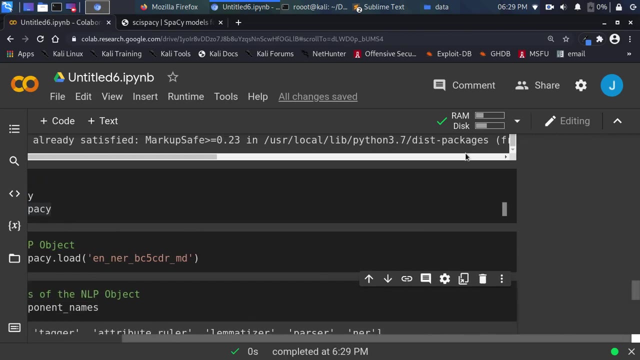 going to be the component of the nlp object that we have. so to do that, we have two ways we have. can just go with nlp dot component names, right, which is a class attribute. so now we can see all the various components we have. we have the tokenizer. let's make it smaller. 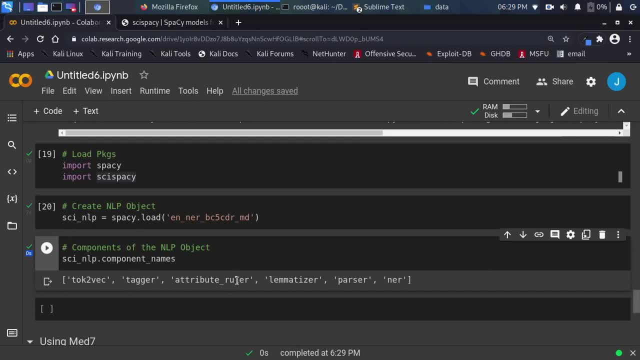 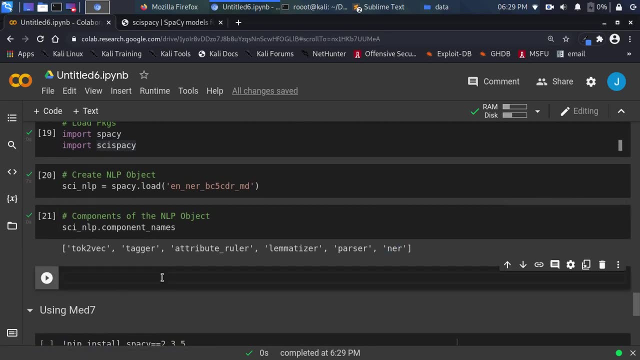 we have the tokenizer, right. we have the tagger, we have the attribute and ruler, limitizer, parser and then the ner. this is the most important thing for our test now, right, okay, so let's first of all, in case i also want to see all the various entities for this one, i can also come back. 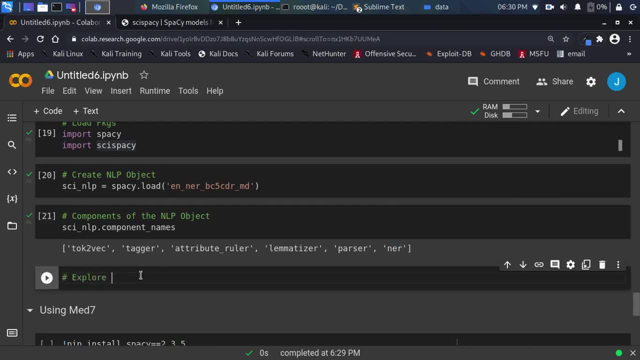 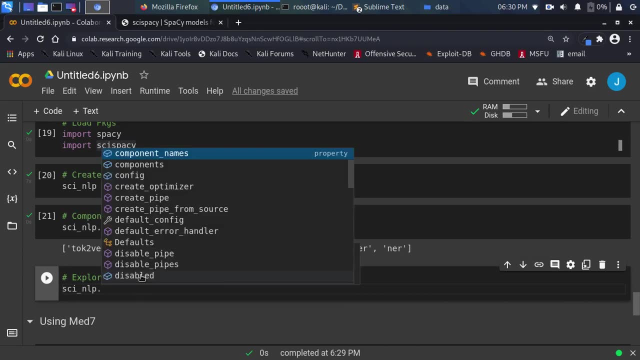 okay, so let's explore the entities. so entities today. this day is going to be my psi, nlp: dot, dot, get pipe right, and then we are going to be picking this in here. that's what you're picking so anywhere. so get pipe in here and now i can just give it. dot the labels, right, i go. 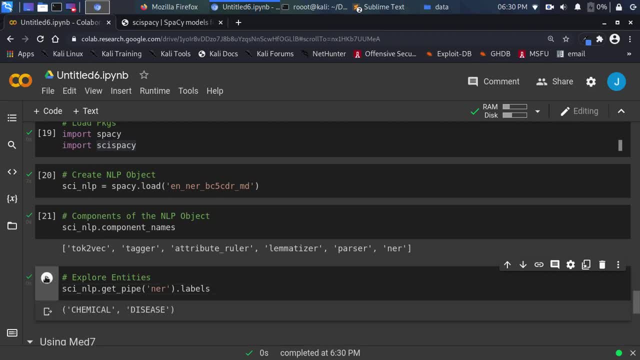 with this. it's going to list the various entities within them, so you only have two right chemical entities, because the model is what bcdr- chemical and disease relation. so that's what you're trying to be picking. so it will only detect chemical which is drugs and disease. 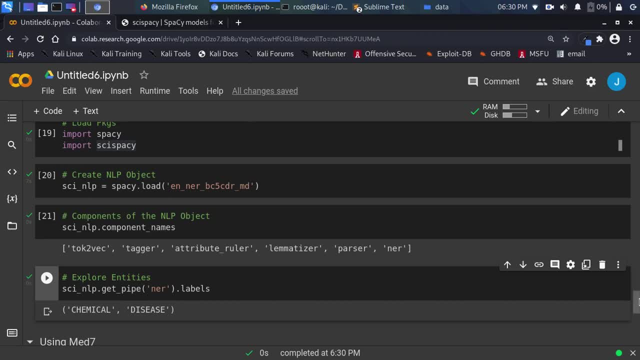 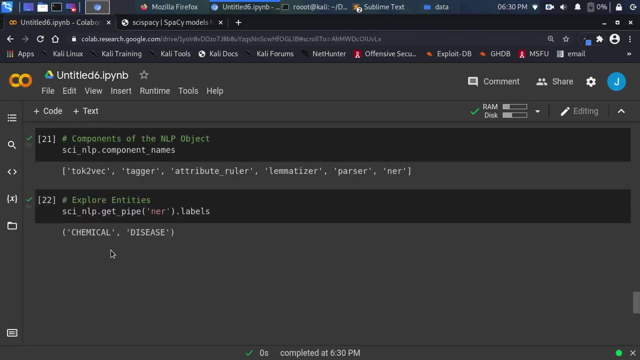 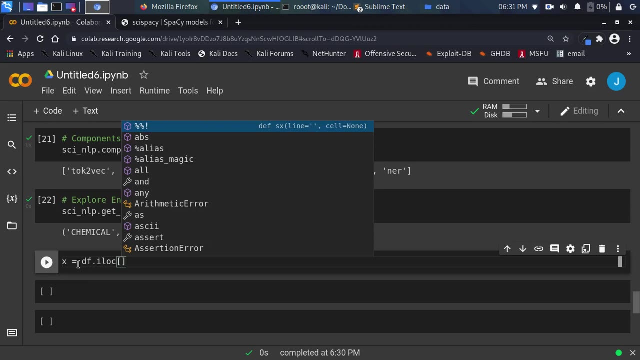 in case you want more, you can use a spark. no, you can use a different pre-trained model. So let's use it on our test. So we didn't not test, So we have a simple test. So let's put example one, then df dot, I look, let's pick example. say one. This is just picking one of 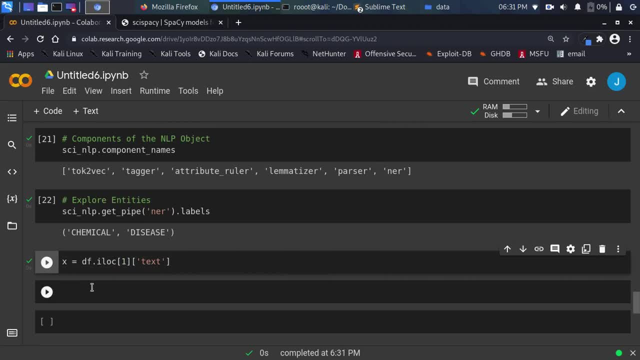 them. we want to be able to see what I'll be able to detect some tests from it, Some of these from this. So let's check this one out. So if I go back and I check it out, I see you have some data. 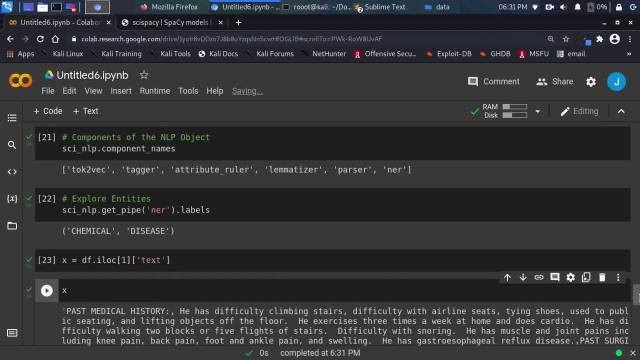 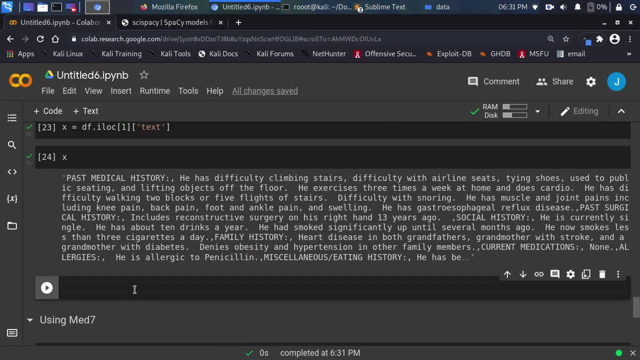 there. Alright, so these are all the data that is going to see what I'll be able to pick all the names and, this day, right, all the clinical terms within them. So it's very simple, just as we do always. So, create our doc, So docs with my sign, NLP, and I'll pass in my 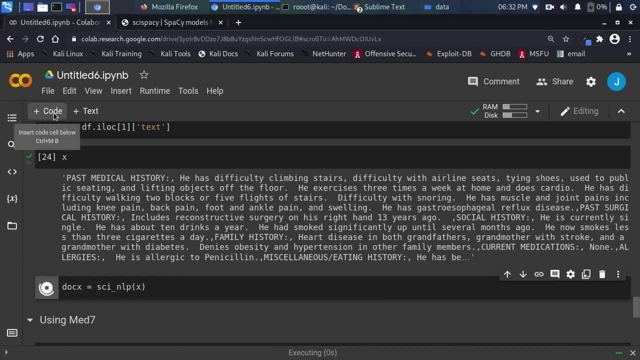 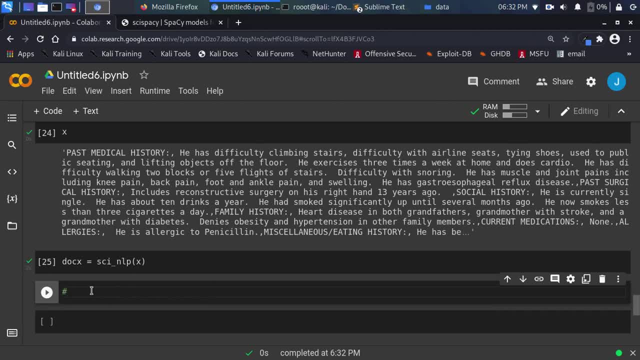 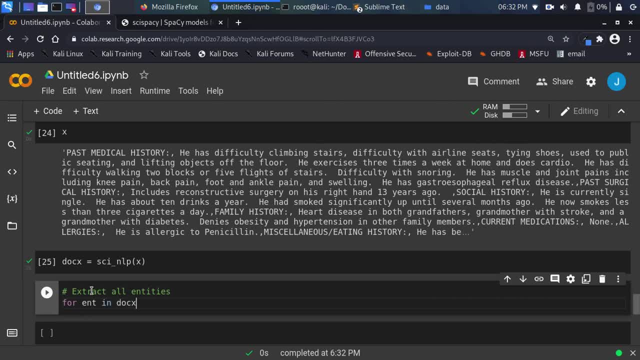 just go with this. So for entity in my dog dot nts. Right, I want you to print all day. See what I did: Print all the entity dot the test and then the entity dot the label, Don't forget. 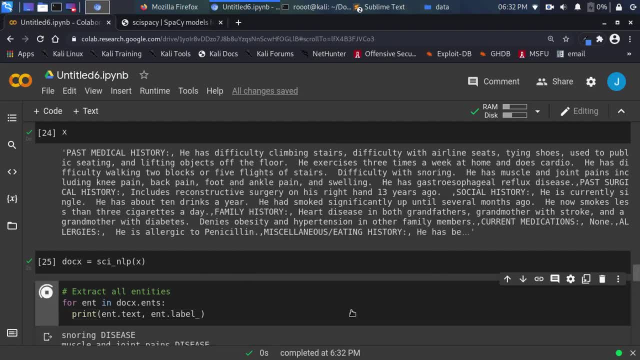 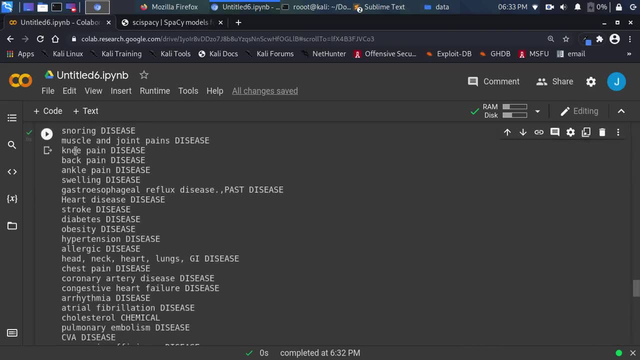 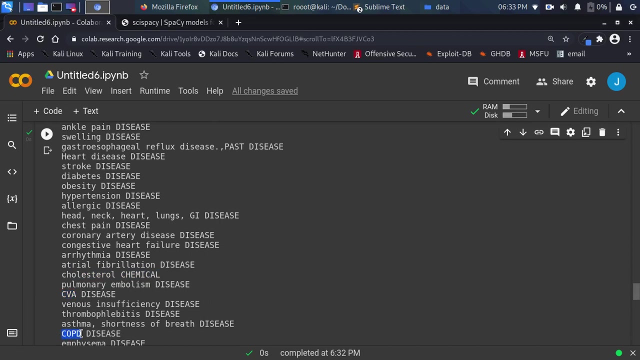 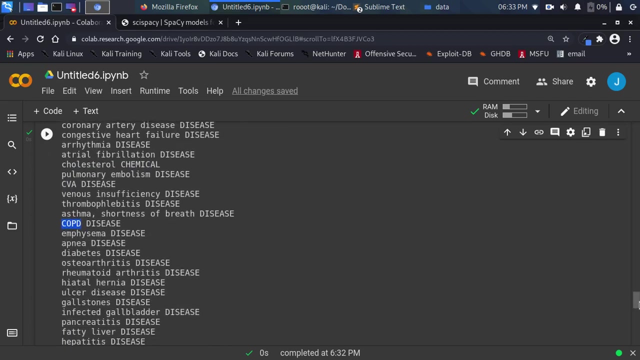 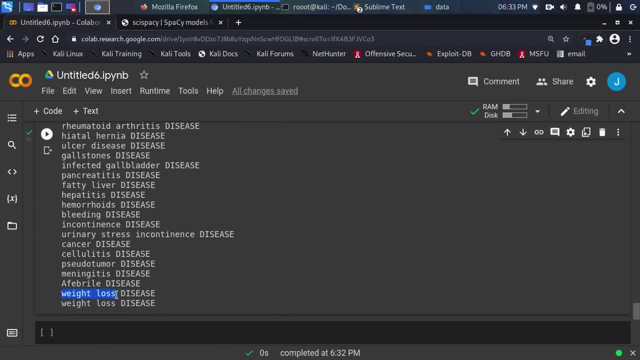 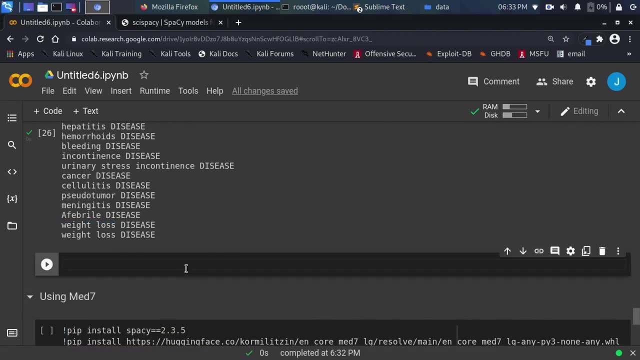 that means is very good. weight loss is not a disease. it can be a, it's a sign, but here we still keep it under under disease. okay, so let's see how to work on it, right? so let's see how to visualize it. so he's going to visualize the entire. 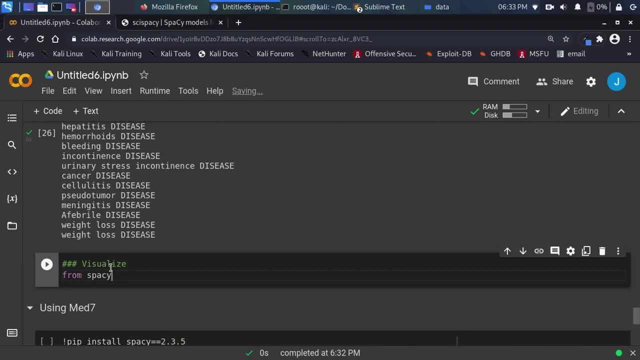 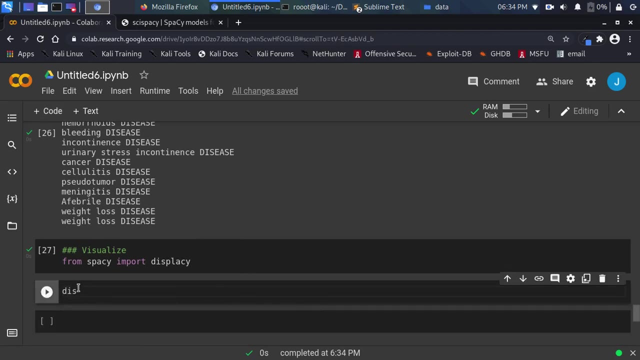 stuff to make it easy. yes, use devices. so, from Spacey, import this play, see right. and then you've been this place II to visualize the entire stuff so I may change the team to make it easy for you to check. so this pleasy that render I'm. 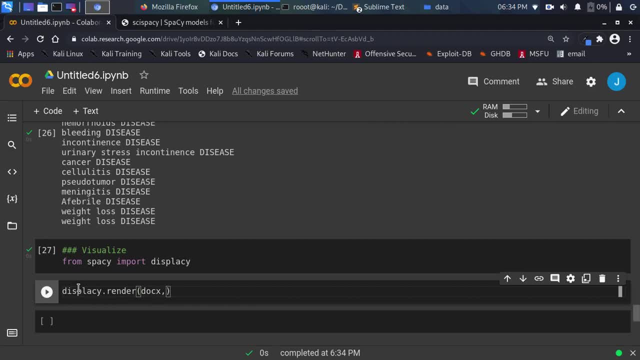 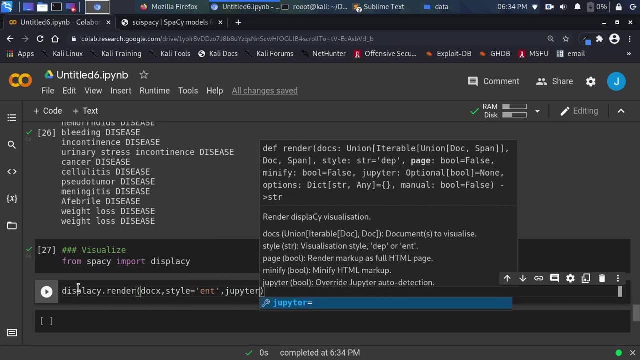 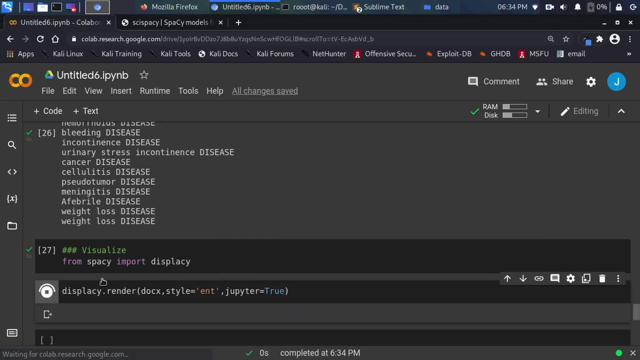 passing mine, docs are passing the star that i want it's going to be ends. and then let's specify that we want to plot inside jupiter, right? so jupiter is going to true, so let's run it. if i run it now, you're going to see the entire entity state right. very cool, just able to identify all the disease within them. 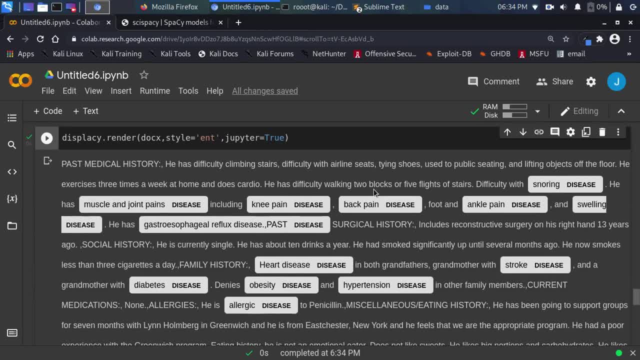 so we have- uh, he was difficult working, he has difficulty working- two blocks of five. you've got two. it's snoring, wow. so all of them. it has been able to identify them, including some of the diseases. it doesn't need to identify penicillin, maybe because of the 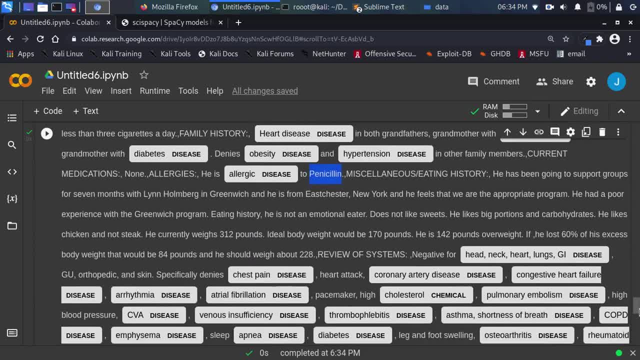 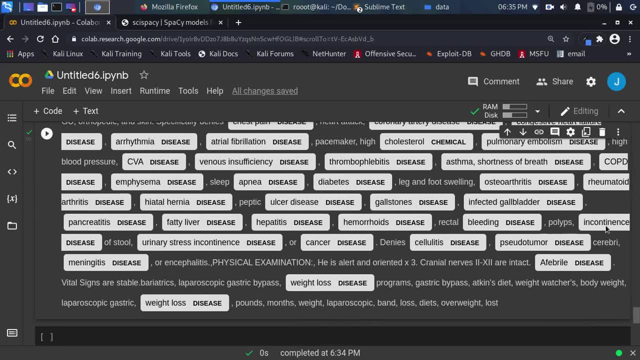 spelling and because of the radiation, but it's able to identify many of the diseases within them, right together with some drugs, some chemicals, right. so let's see perfect. so that is one of the very cool stuff you can. of course, there are a lot of things you can do with it. you can also do: 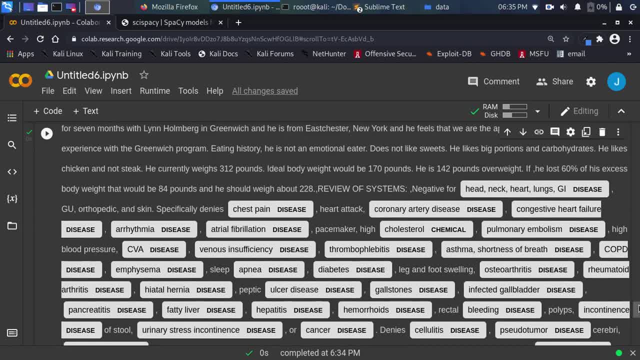 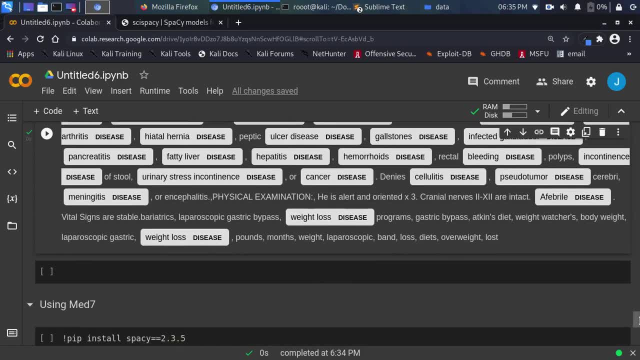 for the dependency parcel and the rest. right, but that is something very cool. based on this model, you really have disease and chemicals, but you can work with other models and get more from that. let's try another package which is going to be met seven. so the same way this time. seven depends. 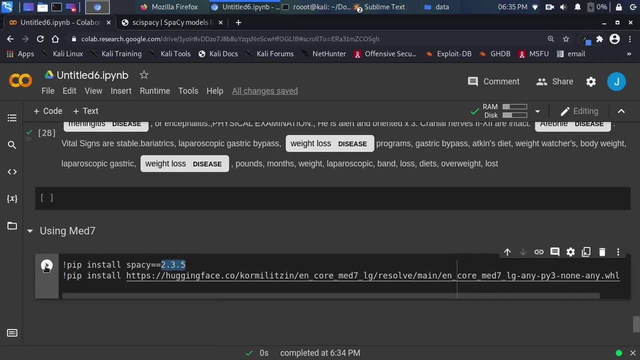 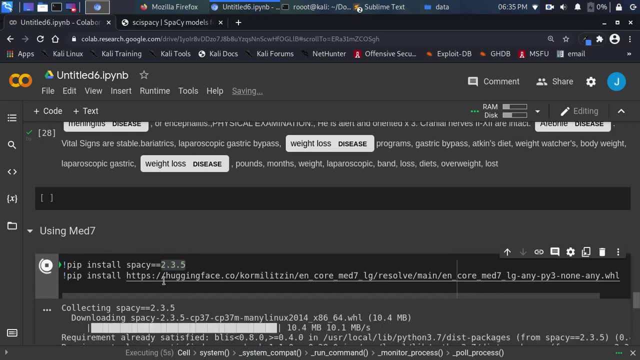 upon specie 2.35. so to work, we just go with pip install specie to 2.35 and then we are using med 7, which is found on hagenfacecom, right? so just going to. this is going to be the url, don't worry. 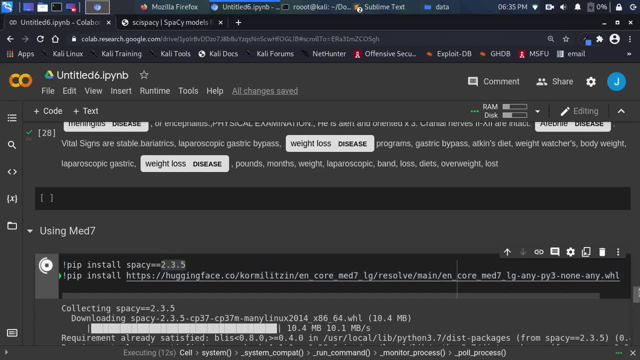 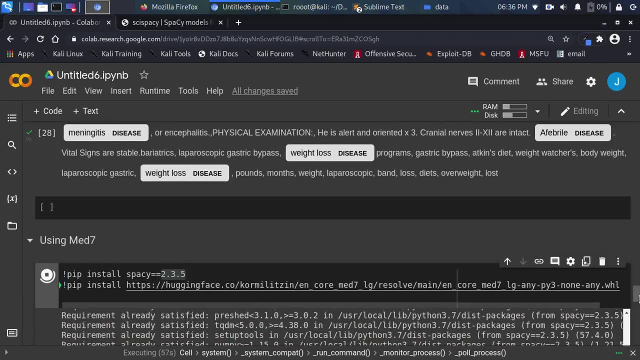 about it. it's going to be inside the notebook so i can also check it out, and then we'll be using med72 also do the same thing we did above. right now, whilst it is installing, let's see what we do. so it is still installing them. it's going to tell me to restart the entire stuff. 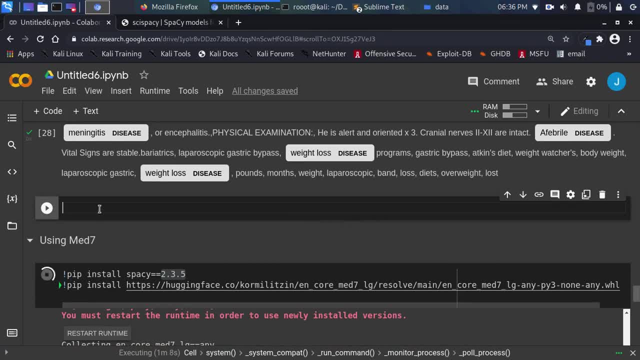 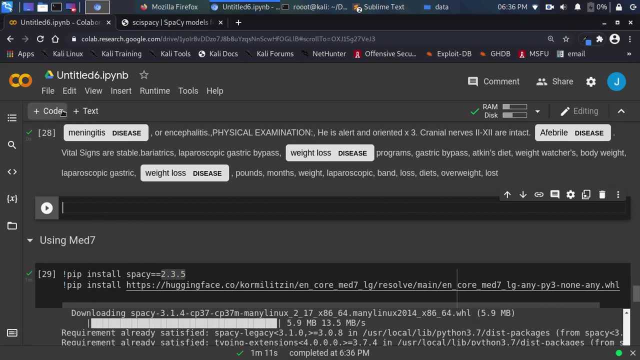 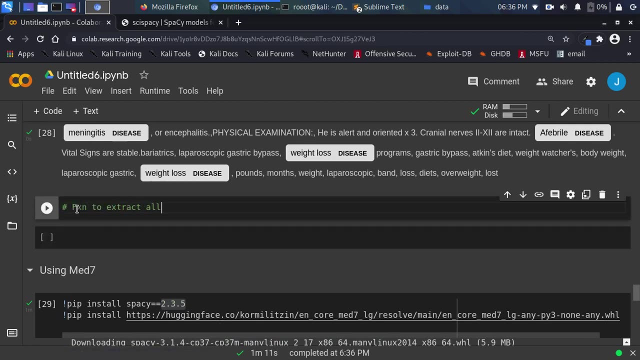 so we will restart it. but before we work on this, we can also create some functions to extract all the disease from our data sets, right? so let's see how to do this. it's going to be very simple. so this is going to be a function to extract. it is to extract all. 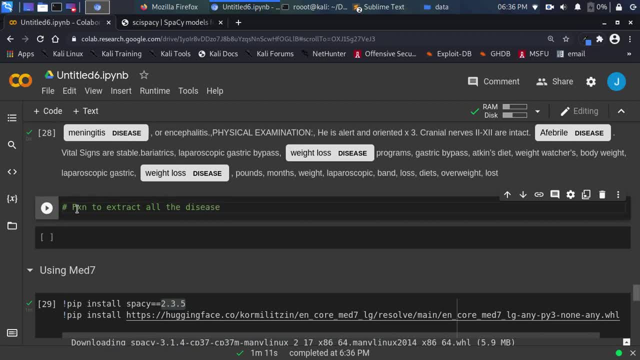 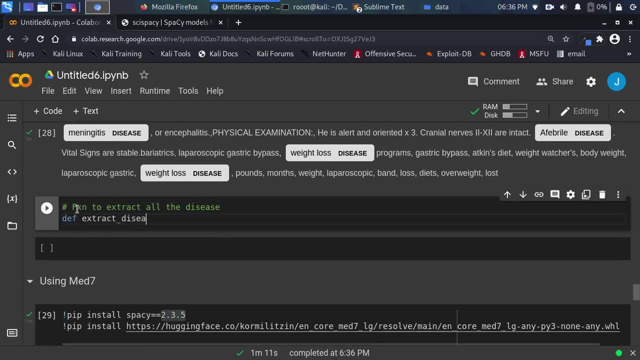 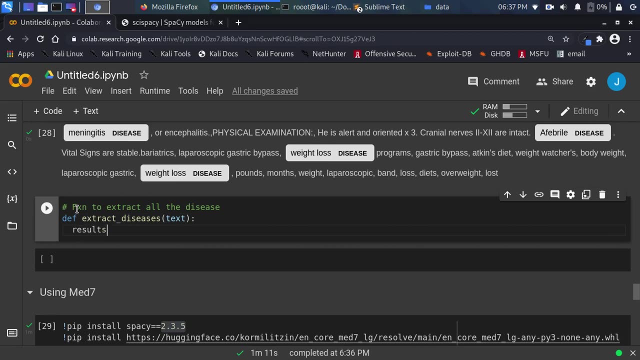 the disease. so it's going to be very simple function and you create another function to plot them. so the function is going to be extract disease. is this right? and i'm going to pass in my test that i want to extract from then this is going to be my results, right? so, first of all, let's 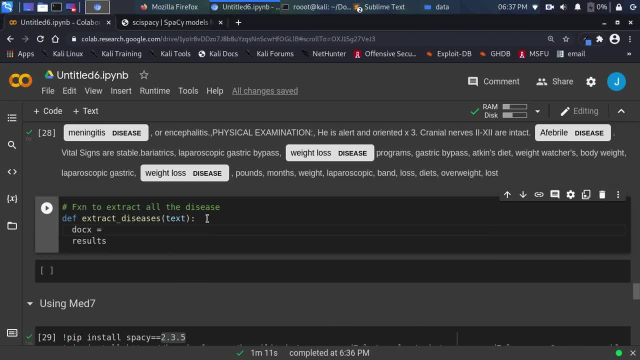 quit the docs, which in this case, is going to be my psi nlp. i'm passing my test perfect. then you're going to get a result. then you're going to say that, okay, entity dot test, let's use a list comprehension. so entity the test, right, let me see for entity. 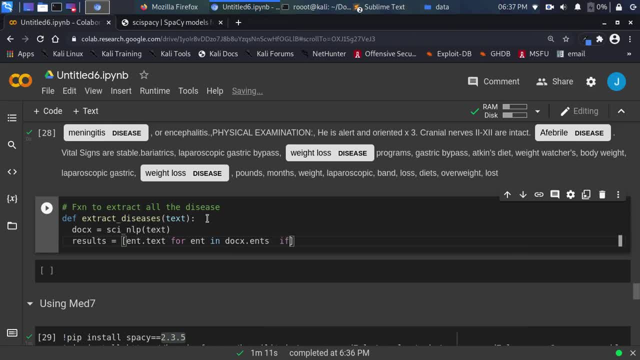 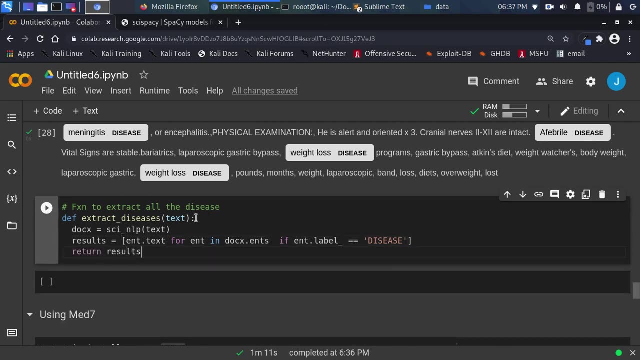 in docsents, just as we did above. if the end t label is equal to disease, right. if it's equal to disease, i want you to pick that one out. so it's going to get the results. so let's return the result. simple fashion we can use to extract all the entities. so, in case i want to extract all the entities, 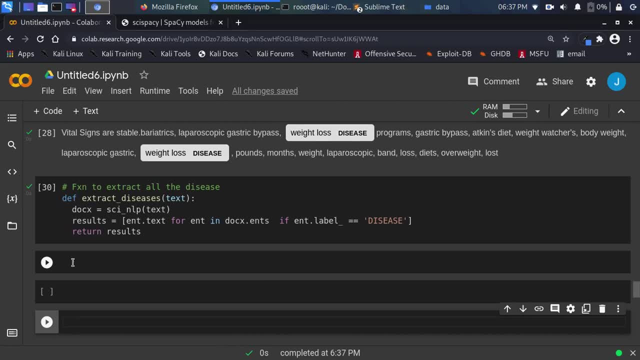 we will do that before we run the seven, so we don't lose what we have done. then i can just go back again. it's going to take some time, right, so i can just pick my data set. so let's go to diseases. then df, i'll pick the test column dot apply. then lambda s extract all the diseases from our test. 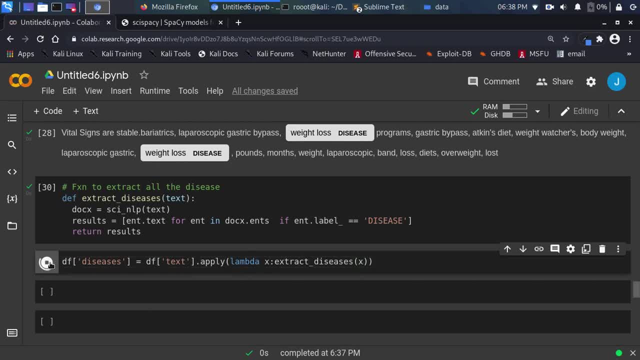 so this is going to extract all the disease from my test. it's going to take some time for it to run because it's a lot of diseases and, as you can see, this is going to be changing because it's going to be spending more information. so once you do that, let's just create another function. 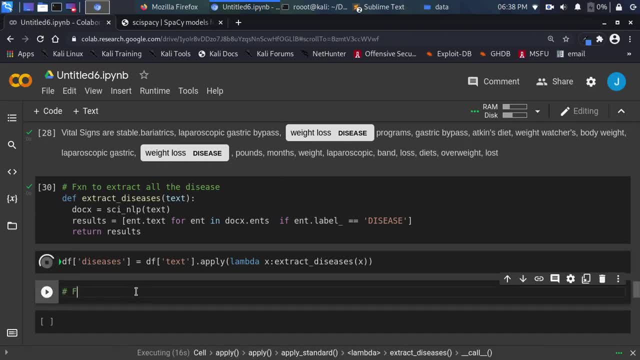 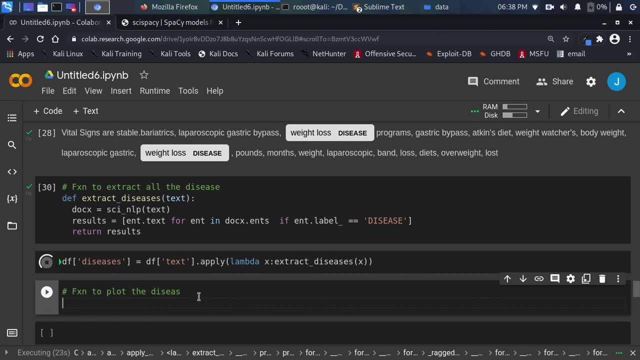 to plot them. so i'm going to create a function, so function to plot the disease right, to plot the commonest diseases. so this is going to be using word cloud. so we're going to be important weight club. so so in case you don't have where cloud is, so i can just tell you just to pip, install word cloud right. 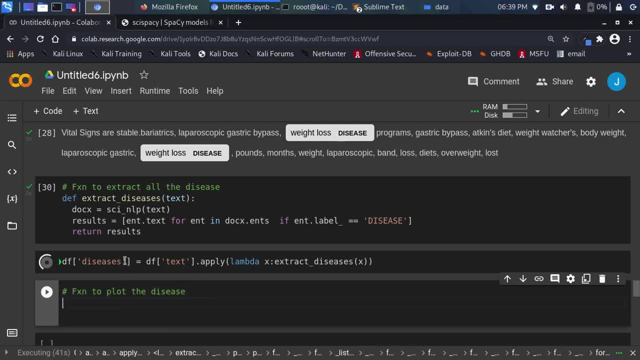 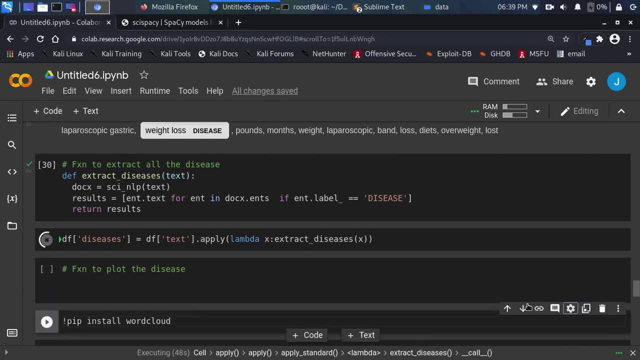 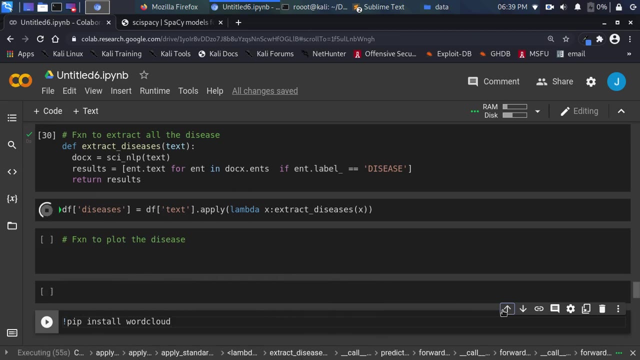 that is how to install this, so let me copy this one and paste it above. so, while this one is running, we will be working on the word cloud aspect. we create a function for a so that it becomes easy for us. so in case you have any question or contribution, you can put. 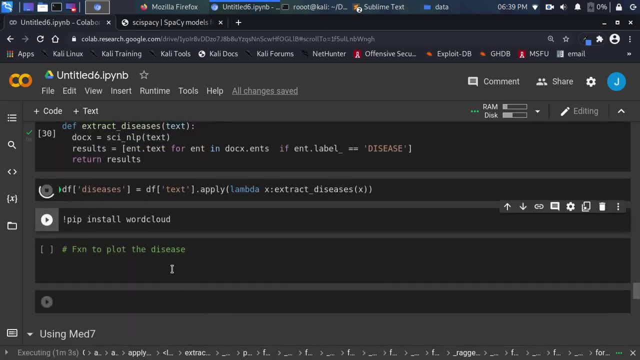 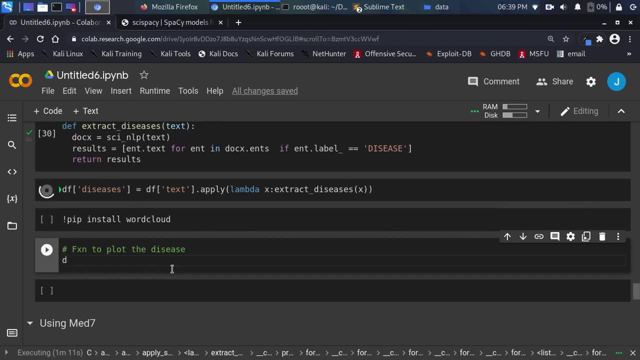 inside the conversation below. so let's go back again to this and let's plot it. so it's going to be very simple here. so let's call it as my def plot word cloud. then this is going to take in my value. so let's call it as my test that i want to pass in. then this is going to be my red cloud. 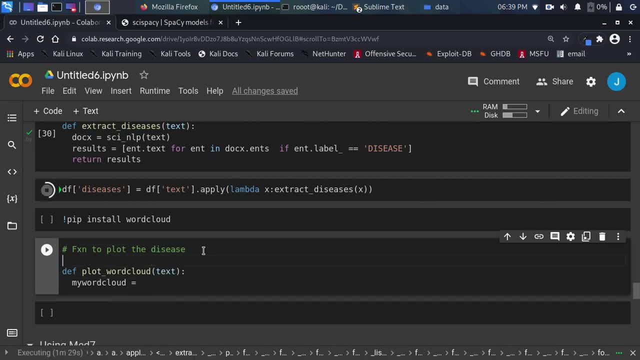 so it's going to take my red cloud. so i have to import it. so it's going to be from red cloud, import red cloud and then i'll pass in my red cloud here. that puts my weight loss to red cloud, the red cloud class, yep. 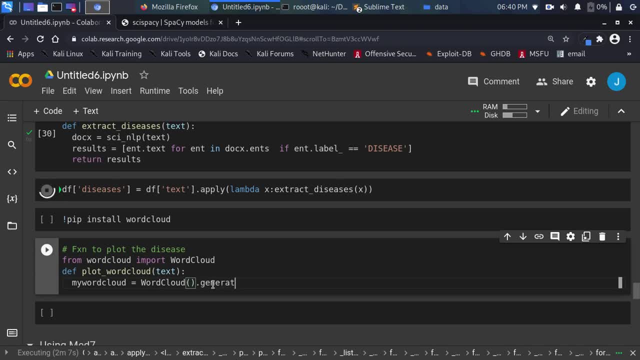 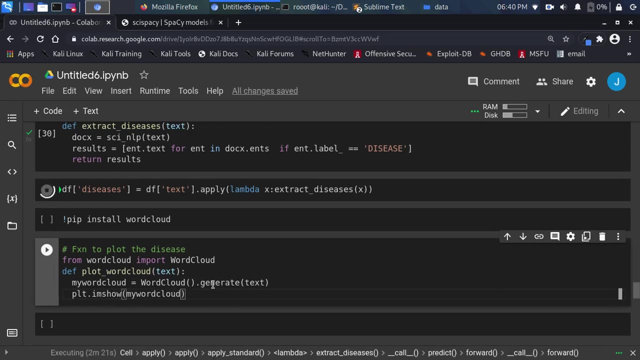 so where the cloud dot generate and then i pass in my test right. so now we can just plot it. so plt dot imp show this can be for mass plus leap and good pass in my word cloud right and then interpolate, interpolation. let's set that one to bilinear. you can change it as you wish then now. 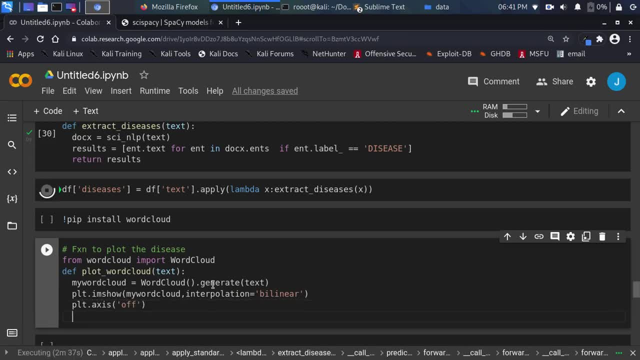 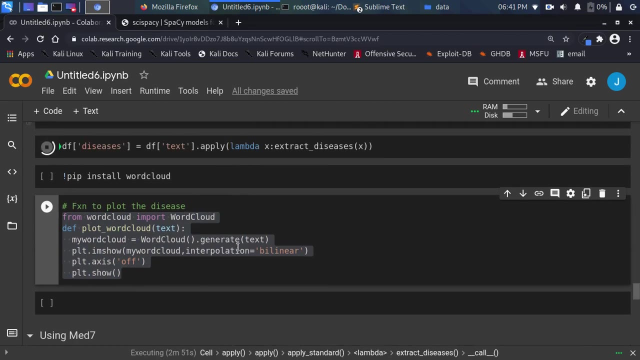 the address off and then we can now show it. so this is a simple function that we have created to help us plot our disease right. the most common it is for a particular test. so while this one is working, what is working, we will just fetch all the g. so, based on the details that we had, 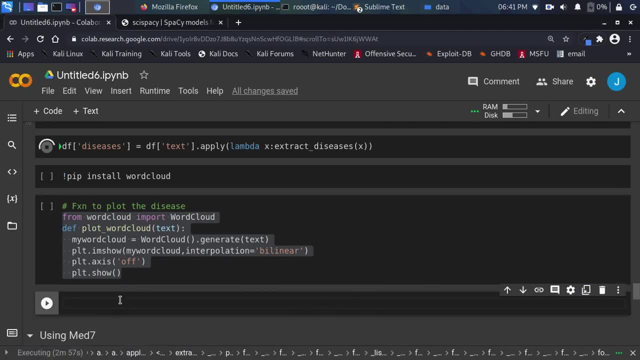 right, we have different labels. so we have three different labels. the df dot labels, dot unique. we'll go with this option. you can see that we have different labels there. right, let's take some time for each one. perfect, so at long last, that's finished. right, that's finished. 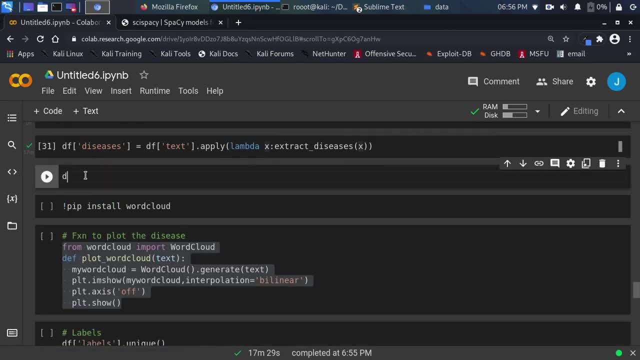 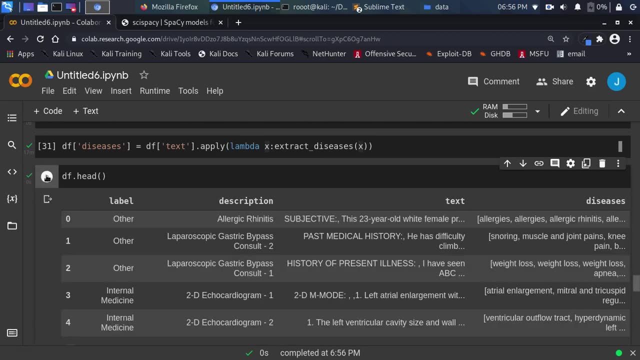 with all of them. so let's go back and check it out. so, df, head and now just finish them right so we can see that doesn't need to extract all the diseases from our test. right, perfect, so we want to get all the disease per the labels and then 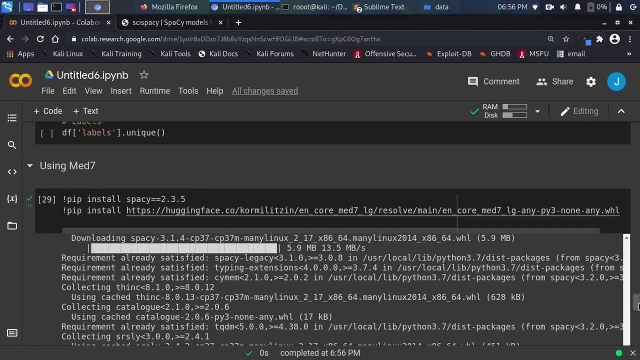 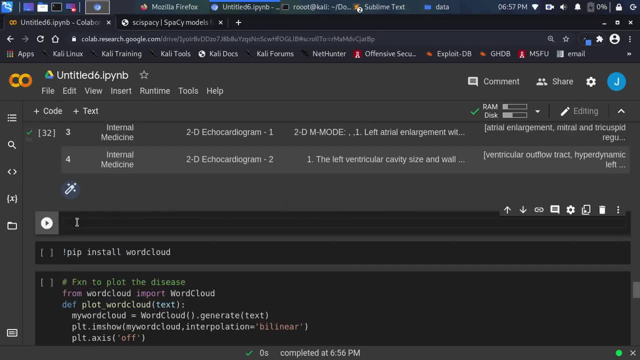 plot them. so how do we do that? so first of all let's go back again and then let's see how to do that. so i just come back to the top of my file and i'm going to create a simple function, so in case i want to get all the disease per label. so we have the label which in: 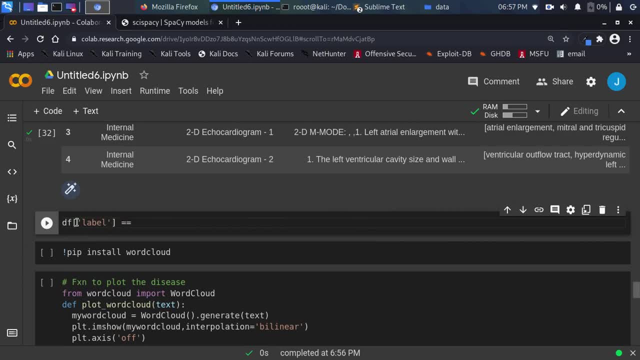 this case we have three different labels. so i want to get the label like, say, surgery- right, because i want to get this one. you can just go back again. so this is going to give me all the diseases that are in the label. so disease, disease or disease? yeah, i think so. so if i run it like this now, it's going to fetch all the columns. 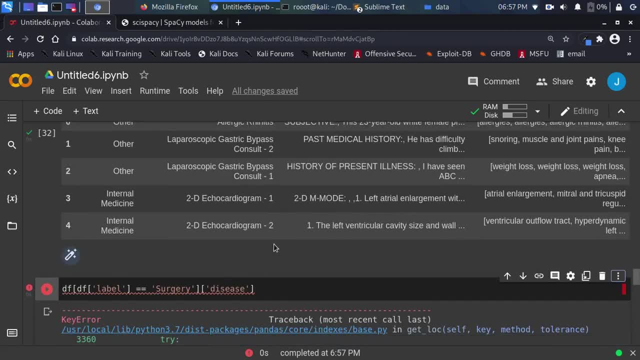 yeah, because i think i made a mistake. it's supposed to be diseases, right? it's going to fetch all the columns that have the label surgery and they're going to give us all the diseases, right. so some of them it's missed because they are not. it was able to find anything and now i can convert this entire stuff. 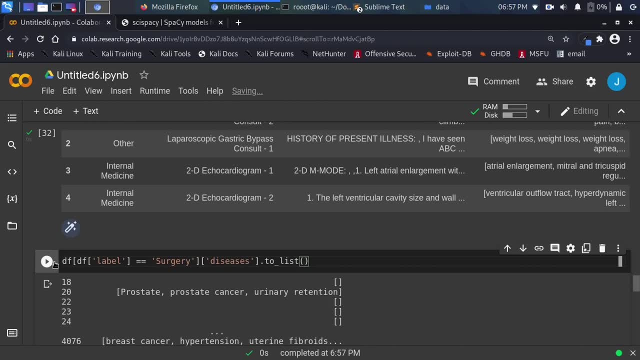 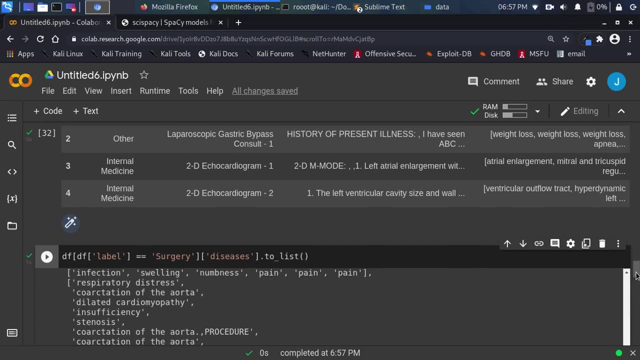 to list. if i convert this entire stuff to list, it's going to convert the entire stuff into a list format for us so we can use it for our plot. but in converting it to a list you can see that it is they asked. it is still a list of a list, right? so we want to take out all of these things. 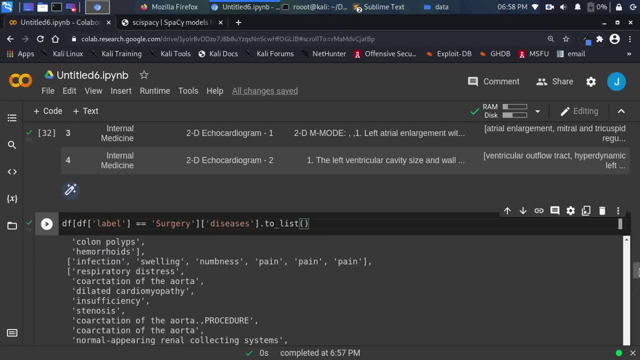 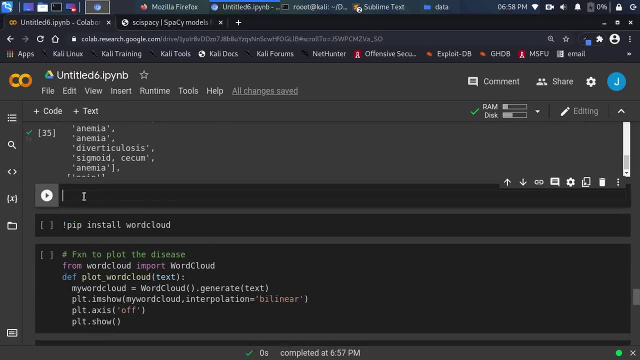 we have to just look through it. so let me show you how to do that. so i've written a simple code to make it easy for us, because to save us time and this is how it goes. so this is a simple function. so the same thing that we have gotten right. you're going to pick the particular label, then i'm going. 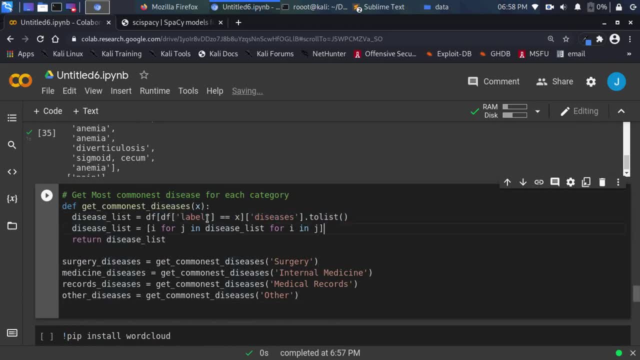 to convert it to a list, as we saw earlier on, and then you're going to look through it to get it as one line right, as one list, instead of a list of a list. so i'm doing the same thing for all of them, so for surgery, medicine, medical records, and then for all the others. perfect, and now we can plot it. 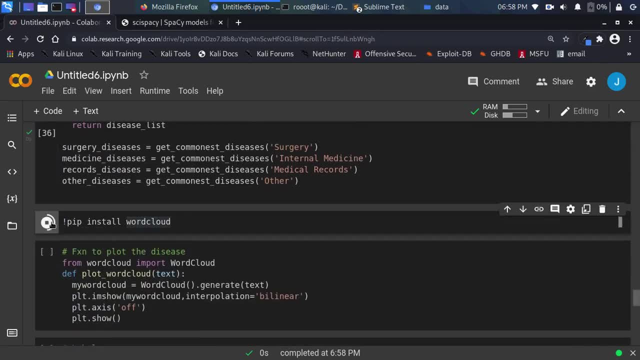 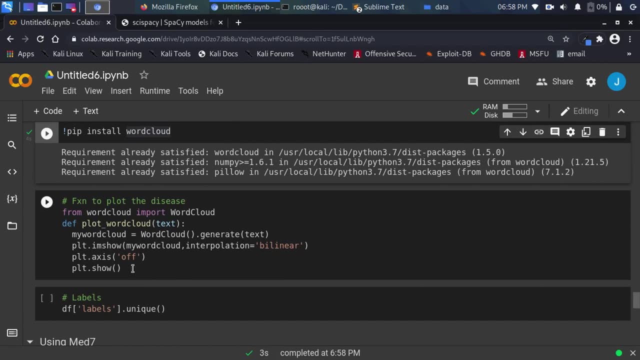 with word cloud. so we want to plot it and see which of these things are so right, so i can now install word cloud and now we can just plug them out right, so we can actually set this size. but let's not do that now, let's plot this, in case, i want to plot it. as you can see, there are three different. 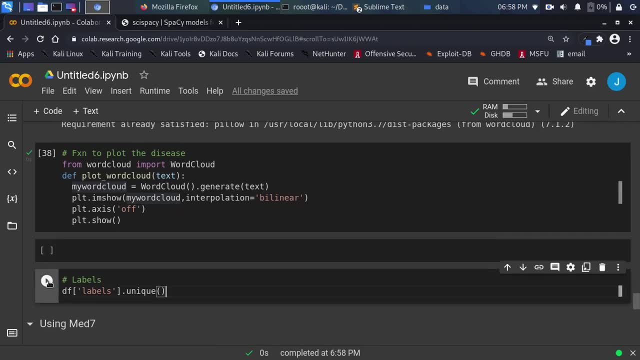 labels. that's why i brought this one here, just to check the labels. there are three different labels. we have this label, i don't know why. today i'm making a little mistakes with the typos. okay, apologies for that. perfect, so we have order: internal medicine, surgery and medical records. 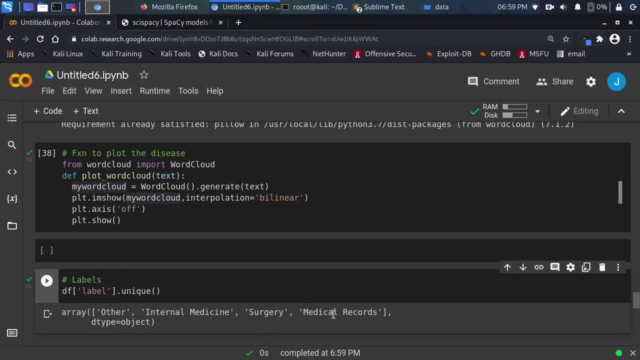 so now i want to plot for only surgery or for medical records, so i can just go with plot word cloud: now passing the surgery right, passing the surgery disease. if i pass inside the disease, it's going to plot all the diseases that are surgery for us. so another error, so it expected. 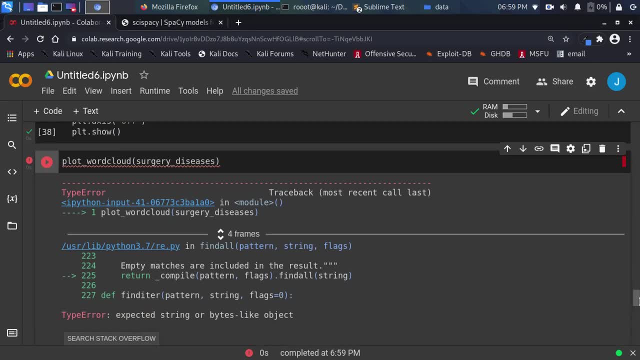 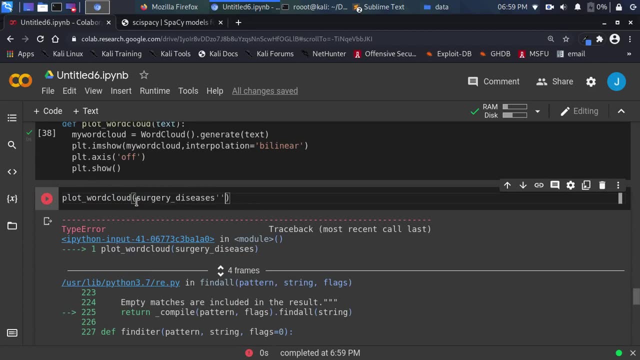 strength right or by string. but it's got a list right because it's a list. so what i'm going to do is i'm just going to go back again and convert the entire stuff into a list, go back. so there's a very slight recall, pretty errors. that makes it easy for you to be able to see errors right in a very 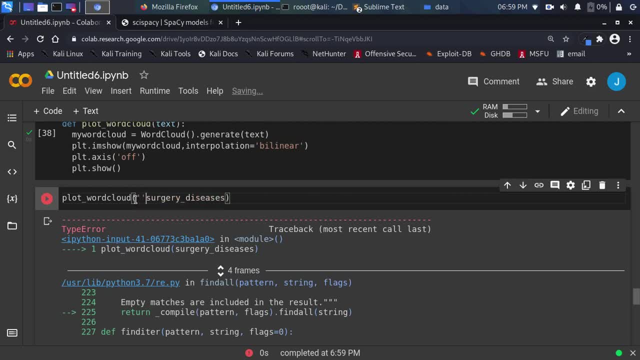 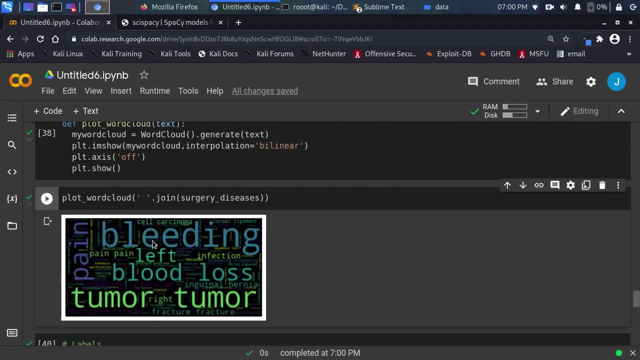 nice way. maybe another tutorial will check on it, so you don't join. so this is going to join the entire stuff as a document for us as one, and now, if i click on it, i can upload it. so surgery: the most important thing for surgery, as you can see, is bleeding. 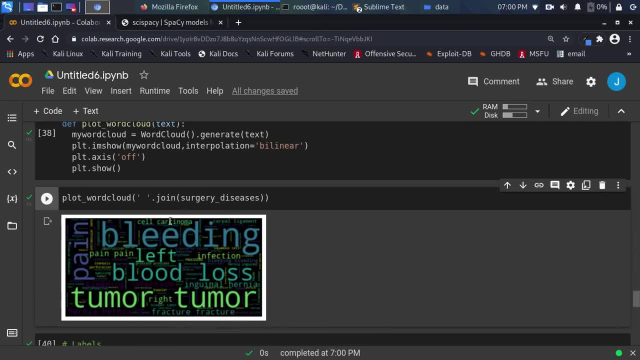 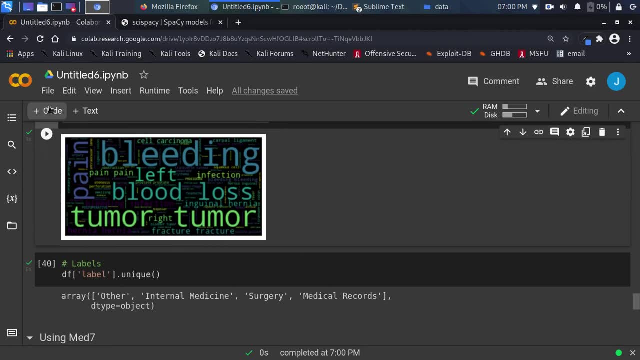 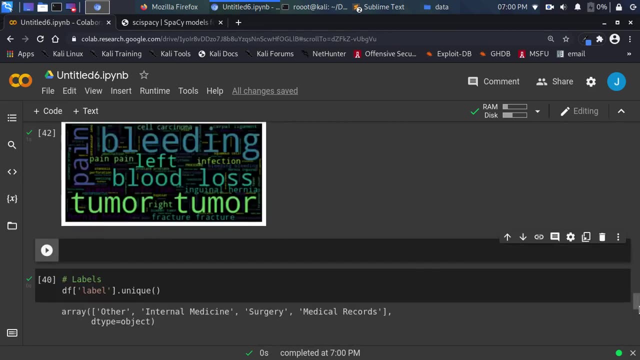 there is blood loss tumor, tumor for an nf fracture, so these are the most commonest stuff there. you can also do the same thing for the other ones, so let me make it bigger. it looks like it is too small for me, or you can make it because you wish let's do another one. so this is going to be what i had here. 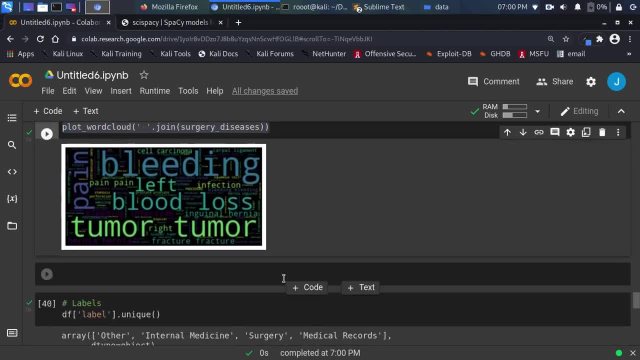 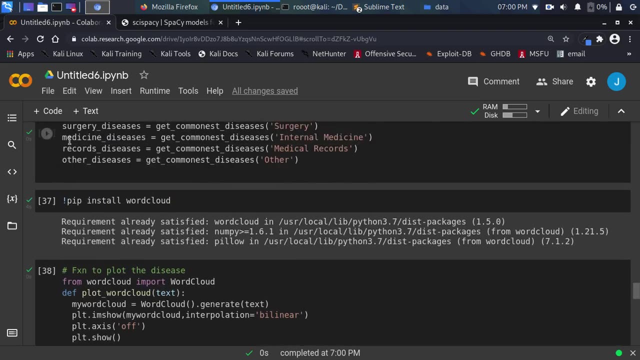 so in case you have any question or contribution, you can put inside the conversation below. so this is going to be okay. let's go with medical, called this medical or medicine. there's medicine records in another. so let's go with medicine and then you just go with the other. 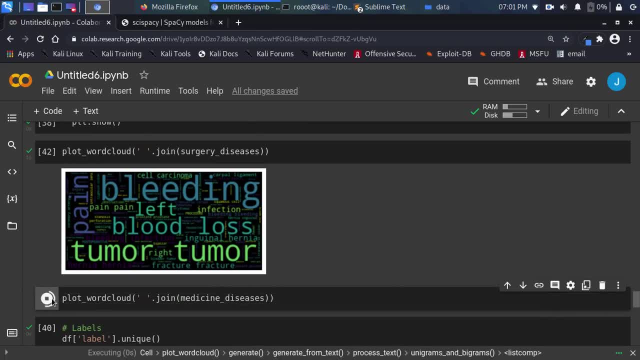 medicine disease. so in america field you have fungal grouping patients. you can just group them according to surgery. if you chest card case, medical a case or medicine case, that is in internal medicine, and then the others right, so you said, for medicine cases or internal medicine cases, you have chest pain, you have alternate cases of chest pain. you 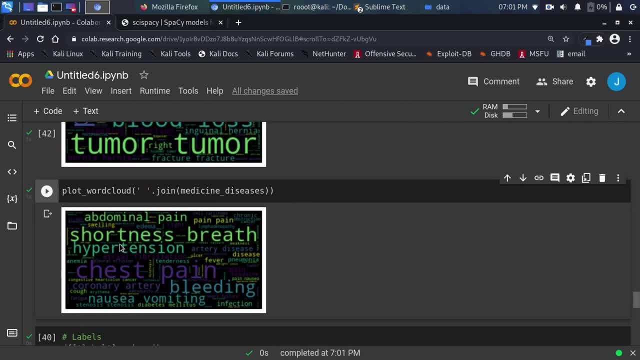 have fenugreek if you say this or it's all way back generation, you can indicate for your patient session. we have chest pain very common. we have shortness of breath. we have hypertension, abdominal pain. know that these are the most commonest cases within or disease within. our data says right. 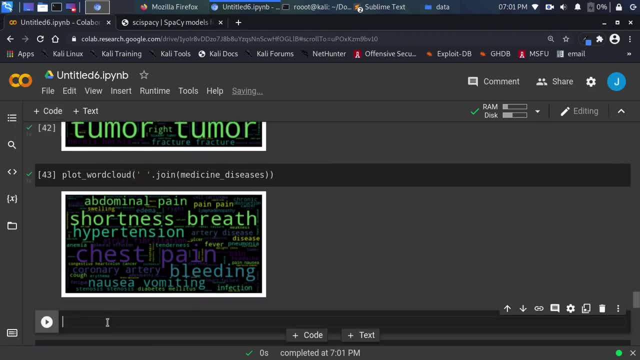 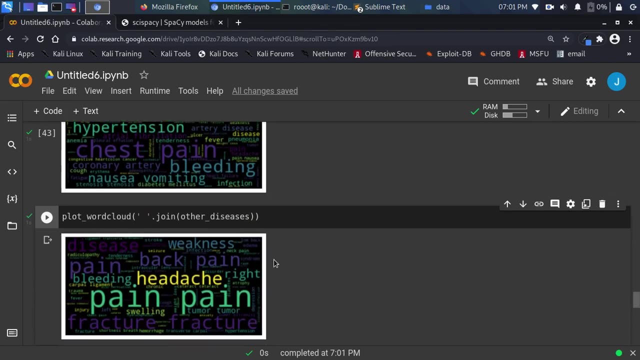 very nice. you can also try the same thing for the next one, which is, in this case, is going to be for the other. let's go for the other, so go with the other. you can now get everything out. so these are the other ones. these are the miscellaneous pain, pain, pain, right, very nice. so now you have seen how. 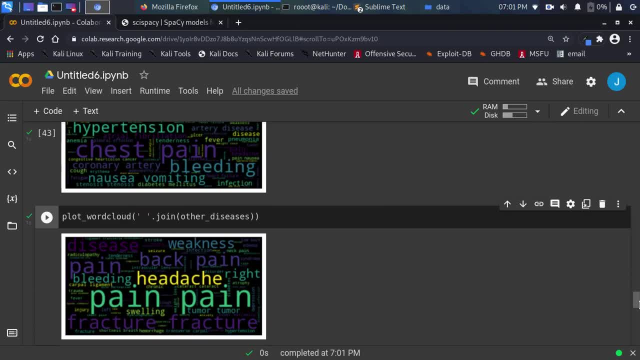 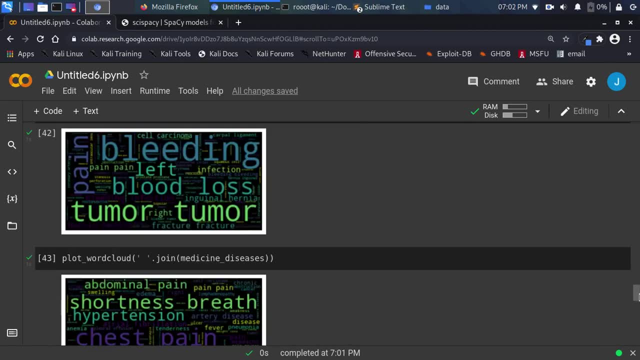 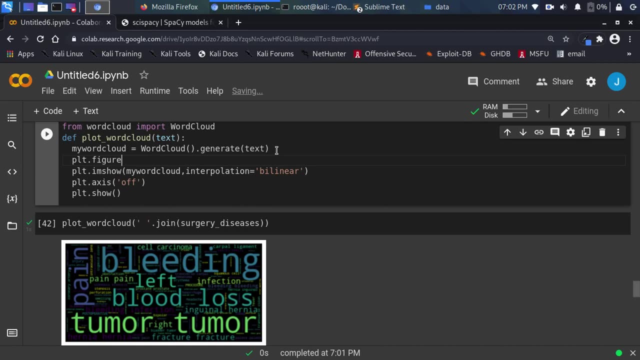 to be able to extract entities from a clinical medical test using size pc and you have seen how to do some simple word cloud plot. you can make this one speaker so that you can see it. in case you want, i can just make it bigger. so this is going to be pltfigure because i want to make 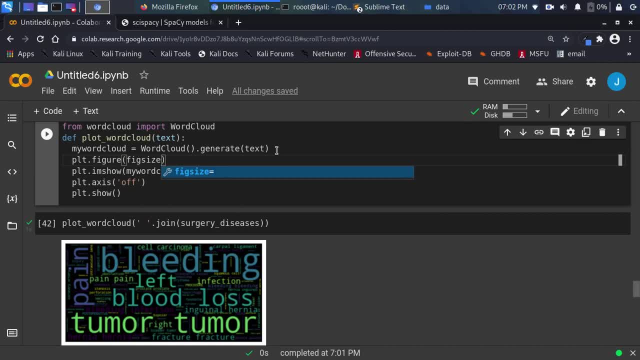 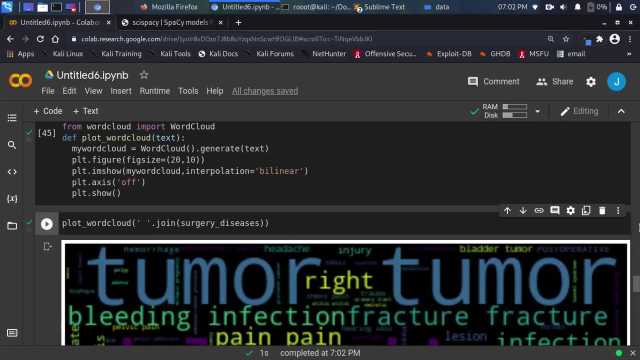 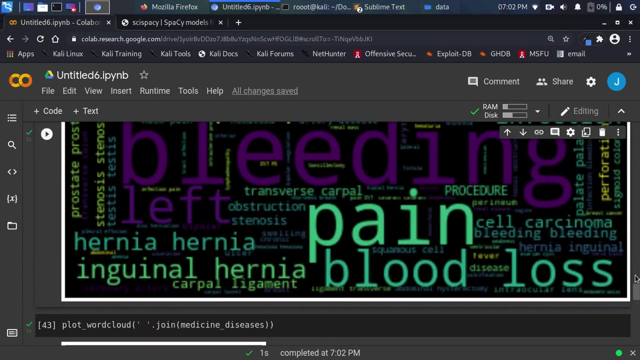 it bigger, then figure size 2010. right, so that i'll. now it is big enough. so if i go back again and i run it, this is going to be bigger. so i can see it. it is big. wow, now you can see the disease you have: bleeding stenosis transverse couple. 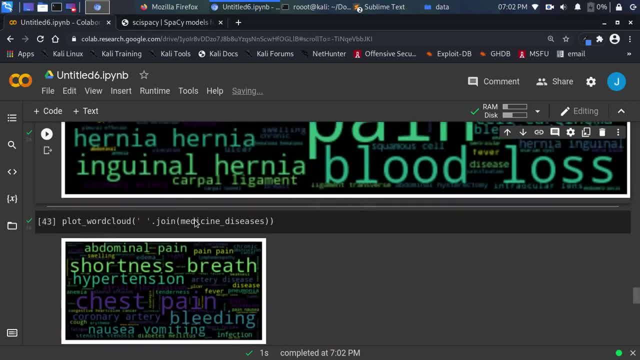 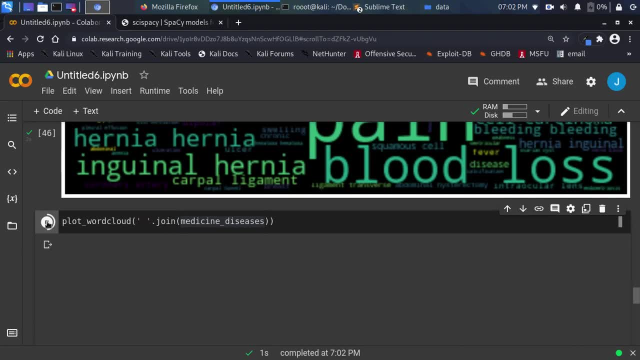 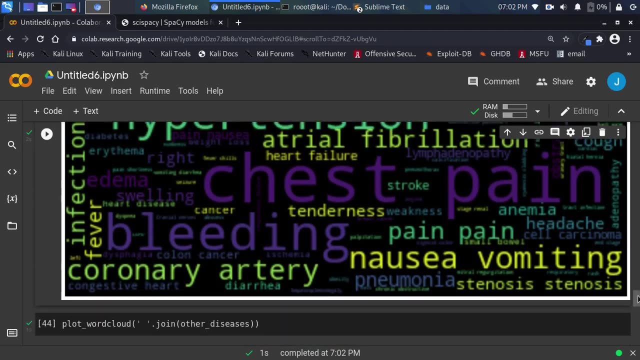 well, very iguana henia. henia is a very common cycle disease radiation, yeah, iguana here in here, abdominal here, yeah, umbilical here, yeah, okay, so we see that this is also very cool, right, which is some very nice stuff. let's try the last one so i can see it bigger. so 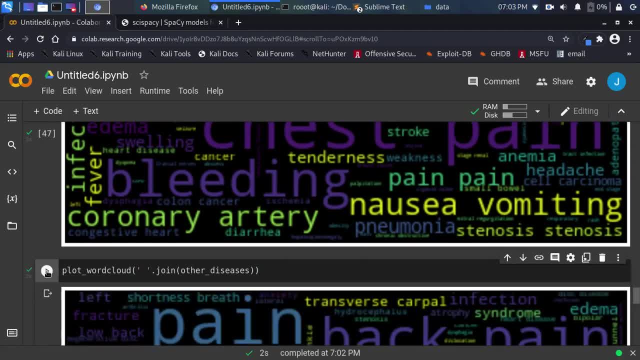 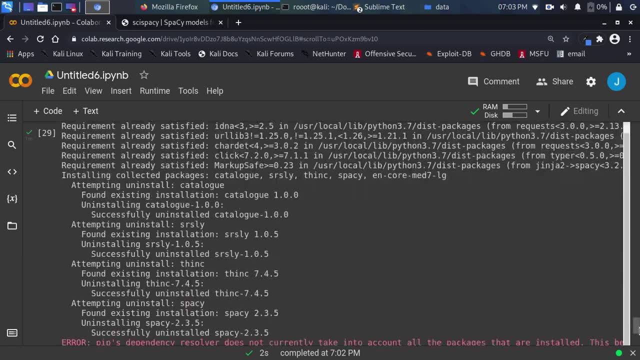 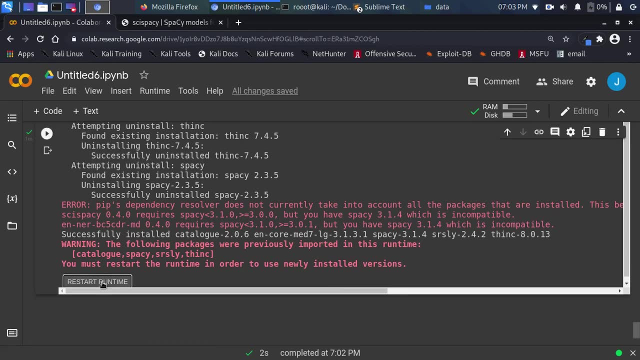 to finish with it, let's end it with the final work, which which is going to be my med 7, right, so within my seven, to help us with that. so, first of all, we have already installed my seven and to work with my seven, you have to rerun, restart the runtime. so let's restart the runtime again, you're. 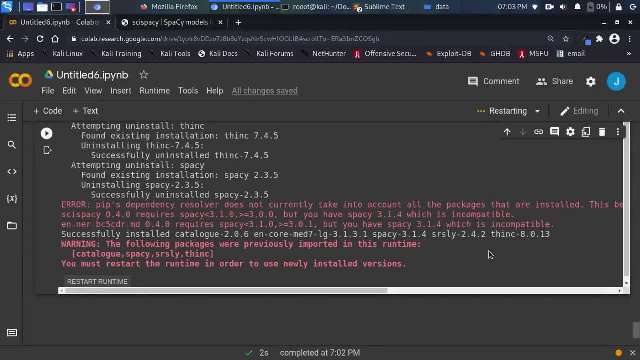 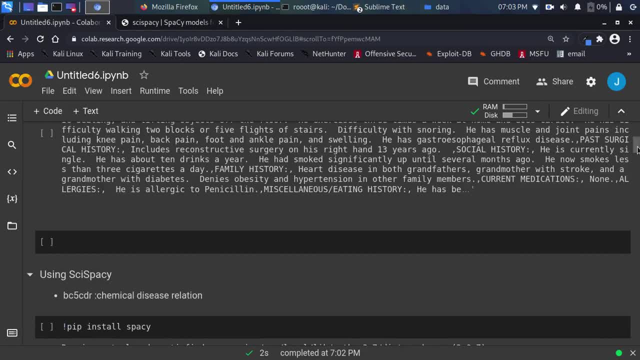 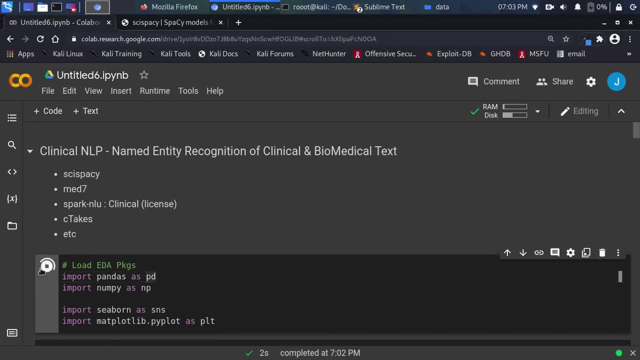 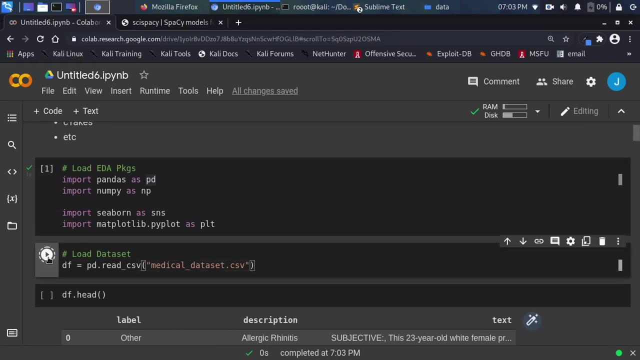 to just finish. if i go back again to the top of my file, i can now start my put these ones and then let's load it, does it and then work on with it with my seven perfect and let's pick the next one, which is going to be my x. 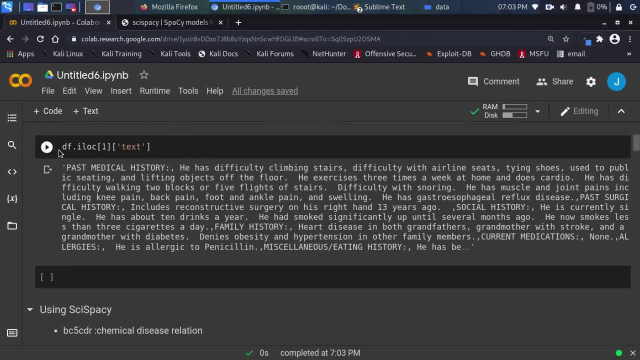 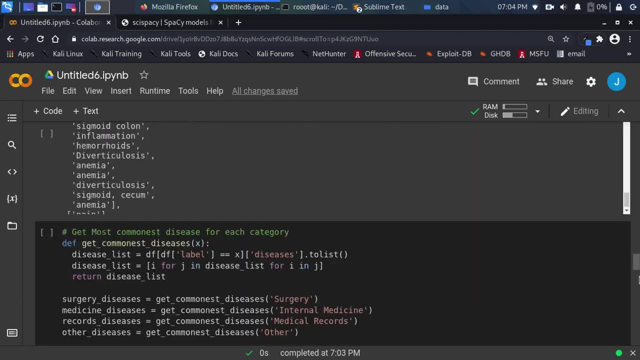 this is the value we are using right, this particular one here. so i'll copy this and then use it to do our analysis, to see if we were to detect the same entities we had when we were using size spacing. so, to work with med7, it's very simple. so. 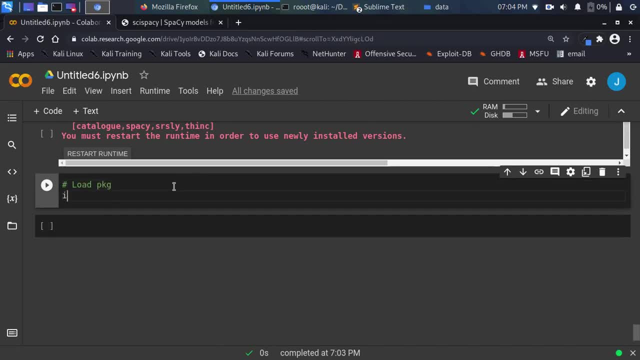 going to load the package, to load package that we import specie right, and then now you can just call: just made seven, so it's going to be specie dot load now passing my med seven stuff. so let me do this one, let's call it on an. 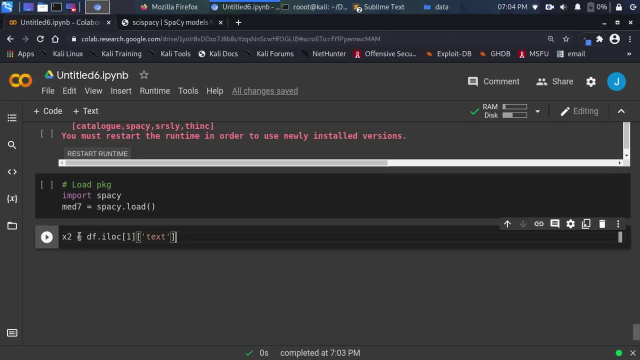 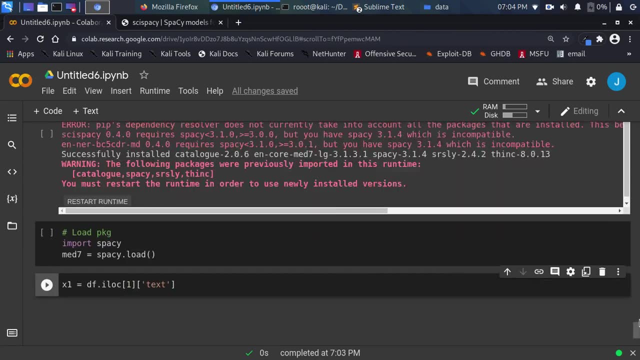 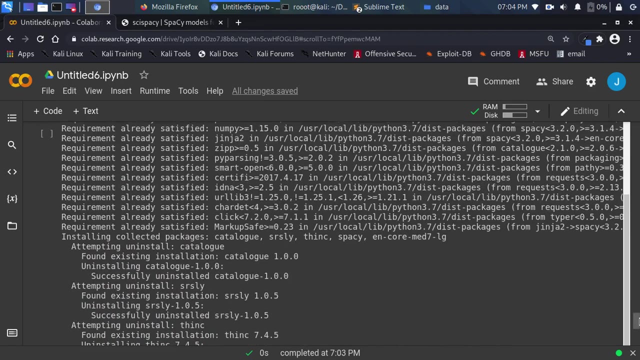 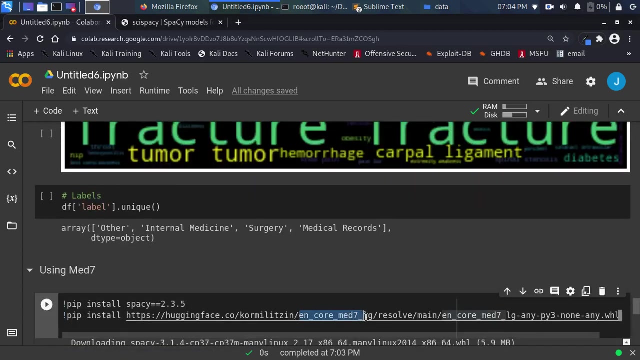 X. right, it's one. so we are going to must pass in the label or the name of the model that we downloaded from this, which is this particular name. here and as we did earlier on, it was underscore, underscore. so let's make sure that this underscore, underscore, which is the same name, so that we don't get an error again. 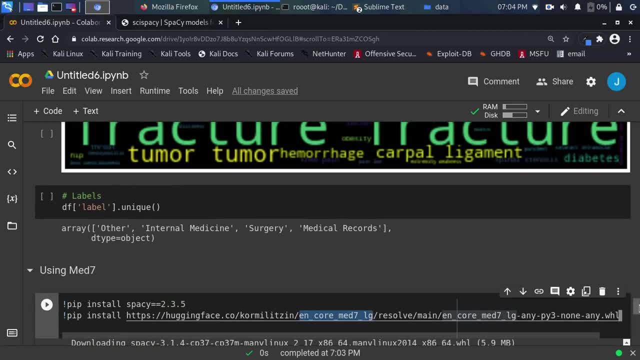 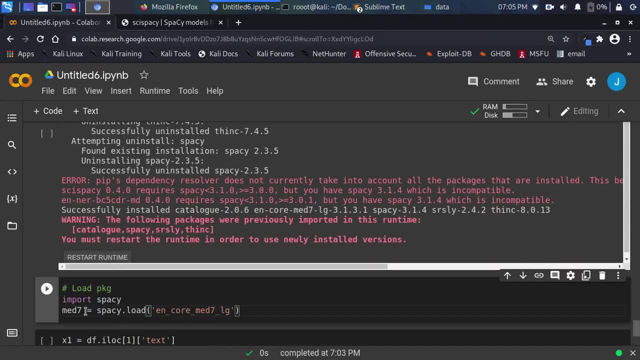 so I'll copy this, which is the name of the model for my seven you and I'll pass it here right, so now you can call it as made seven and LP. right, and if I run it now, I'm going to get it initialized and then we can now do the 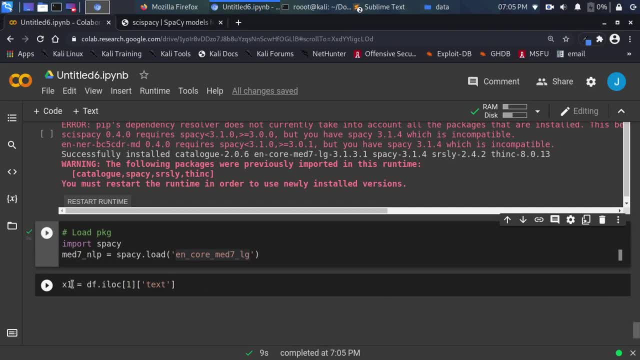 same thing we did previously: perfect. so that's finished. now let's see if you can be able to use med seven to extract and identify all the various entities there. so before we do that, let's check for the various components of this. so let's check for the component. so it's going to be made seven, as you did. 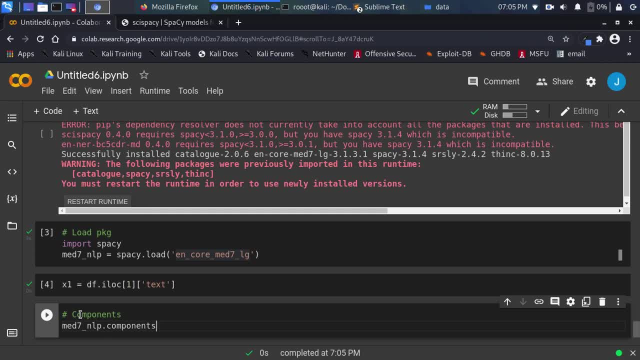 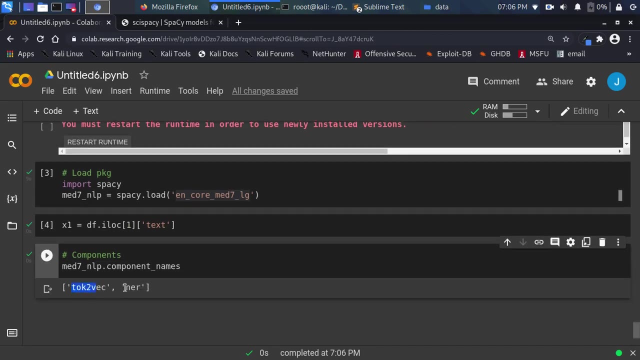 wrong, it just unity. sorry for that because I narrowly and added parent 你是 Hee jagron? yeah, good component names is going to list the component things. so made. seven is very little. I just have the tokenizer and then you're not like nice piece which is having curse IQ tips, the NLPcom and NLPcomponents, NLP, NLPcomponent names. A good component name is going to list the components name. so med. 7 is very little, I just have the tokenizer and then any wow, like Sykes' visit, which is has it having several different component and if I kiss, I want to check for the various labels day. so is good, you may 7. and then we go to alkopi argument Rob, and is going to go to al 9. I mean promotion, ingeneration point. I don't know. most of them have NLP0 component tournament. 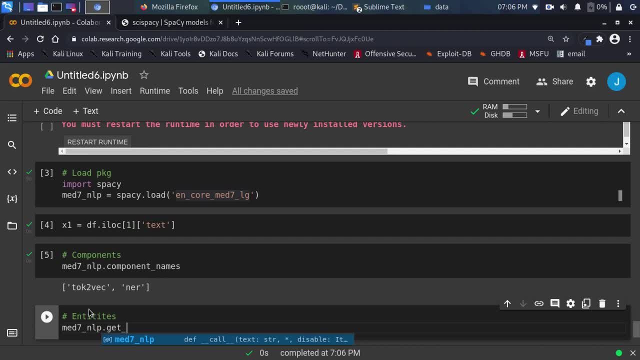 nlp dot get pipe, as we did earlier on, and we're going to get the particular pipe to get pipe, passing the particular component in here that labels. we want to see the various labels there, so to see the various entities that we have. i think it's going to give us. 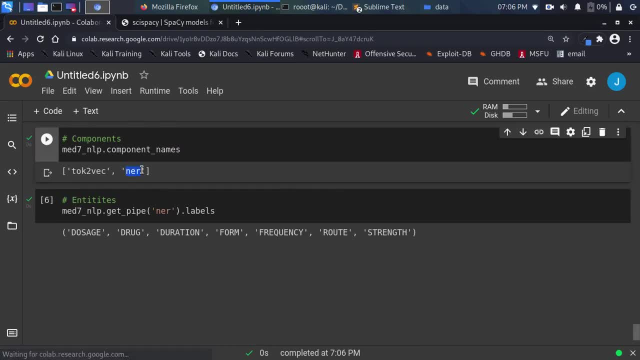 wow a lot. so, although my seven is having just two components, but it has a lot of labels, so we can just check for the usage of the drag, right, you can check for the drag itself- duration, form, frequency, route and strength, which is quite good, but if you're using spike, nlp or spark, 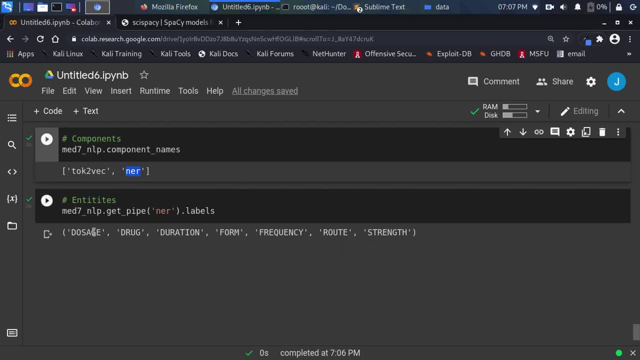 nlu for the clinical version. it has a lot of entities there. it has to say drag duration, negation procedure. that's a lot right. so let's see if we can be able to identify some of them. so i'm just going to pass in the same thing. so let's go to my docs too. so made seven nlp. 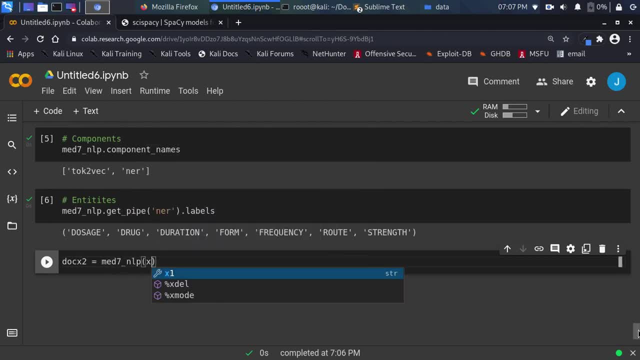 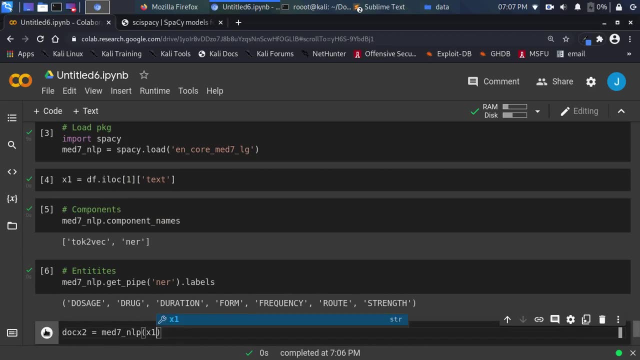 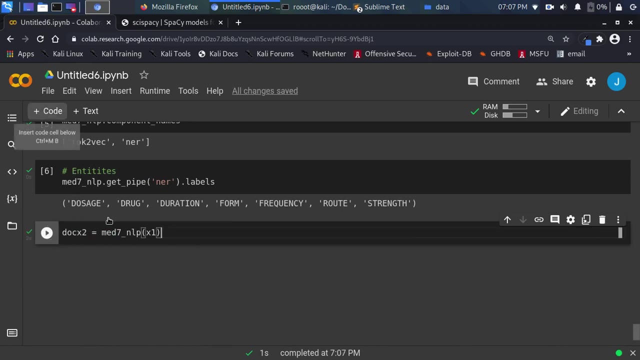 i'll pass in my s, which is referring to this particular value here, so s1. so you run it, and now we can now visualize this. so let's visualize this instead of extracting them out. i'm going to visualize the entities there. so from specie import displacing, and now we can now. 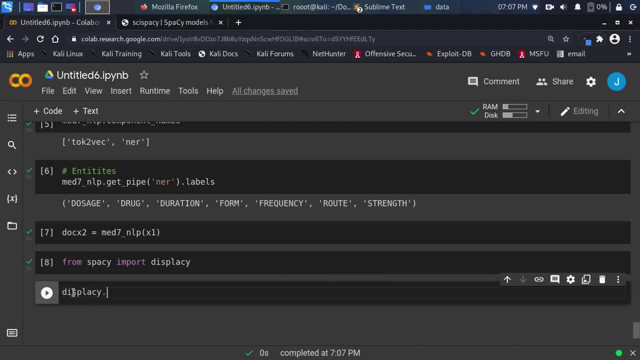 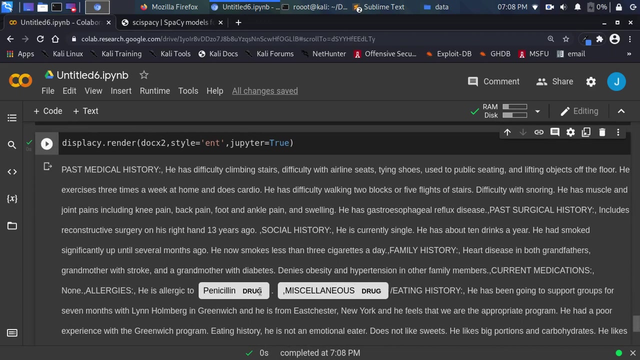 true. now visualize so disp machine see just able to identify, not most of them, well, just able to identify penicillin. right, Unlike the one we did, we didn't identify penicillin. So penicillin is a drug. I don't know why miscellaneous is a drug. 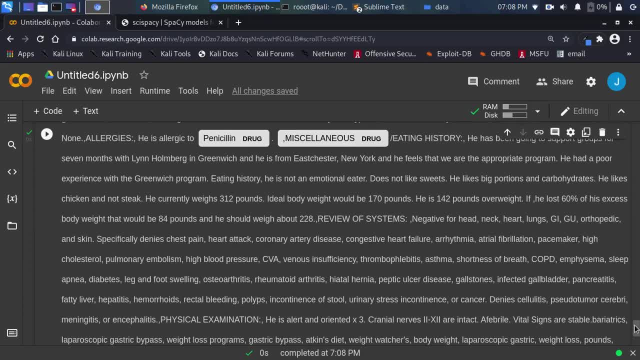 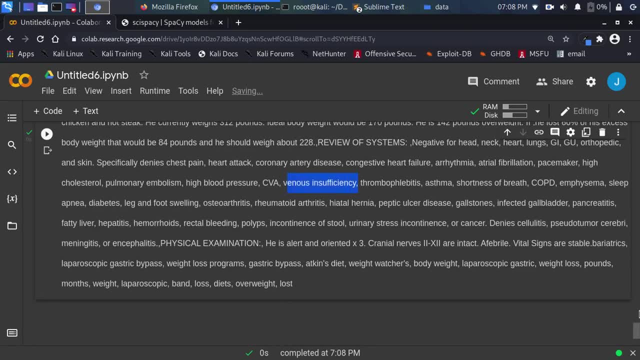 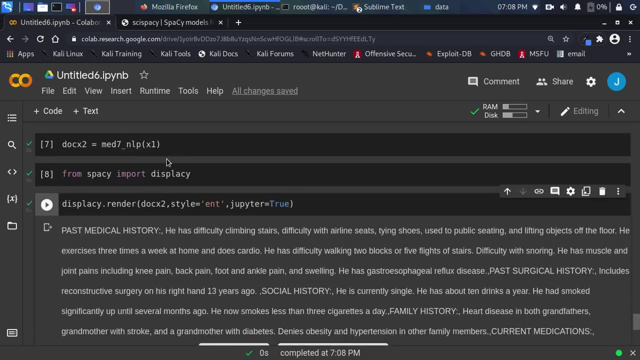 Funny, But it cannot identify some of the diseases. Most of these diseases cannot identify all of these things. It cannot identify them, But it was able to identify penicillin as a drug. Let's try another example. So you have seen how to use Med7 and then Displacy. 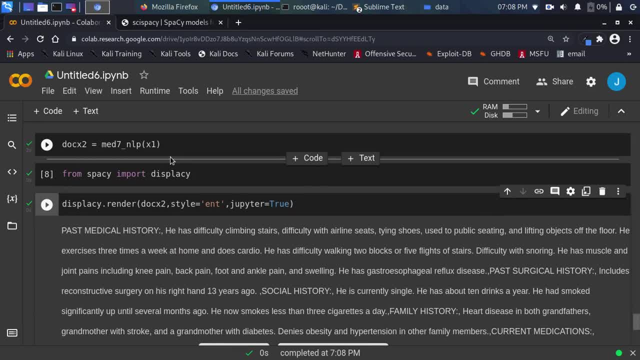 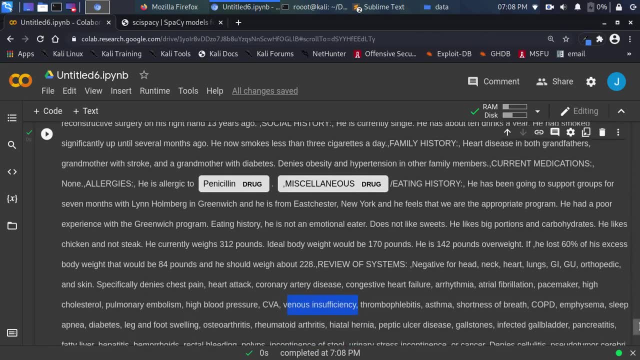 And then CySpace to be able to extract or do named enzyme recognition of clinical test. In case you have any question or contribution, you can put it in the comment section below. We can use this one to do a lot of things. There are a lot of cool stuff you can do with this particular package. 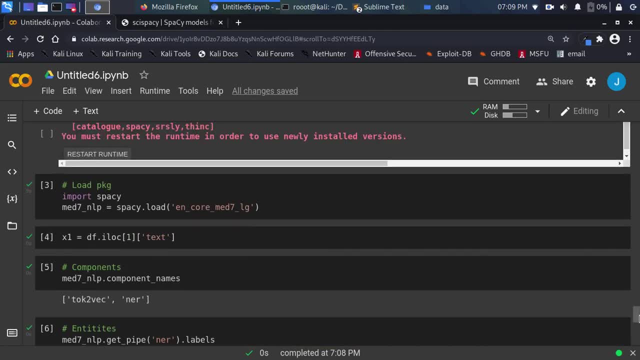 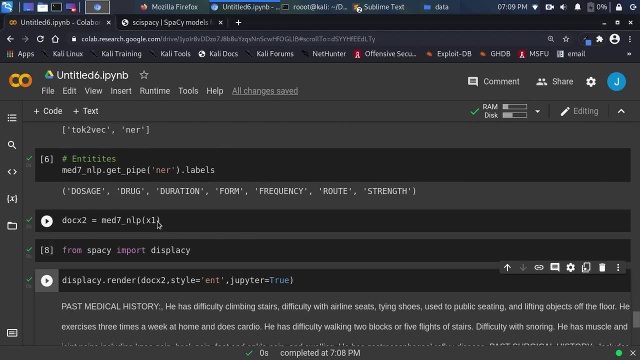 But this is some of them right, Because with Med7, you can see that we can extract a lot of things. So if I had the procedure and everything well structured, I would be able to get most of them. So let me do this way.